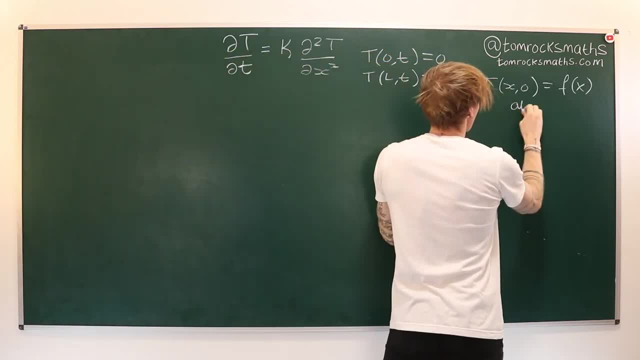 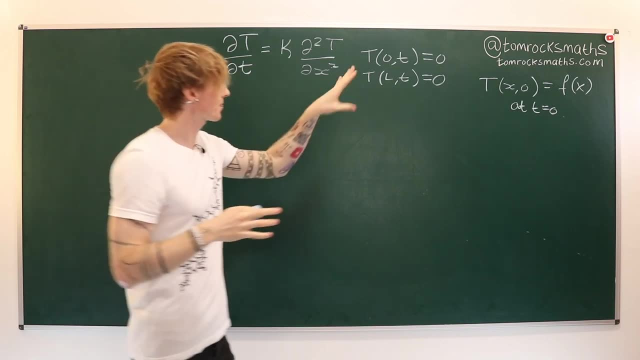 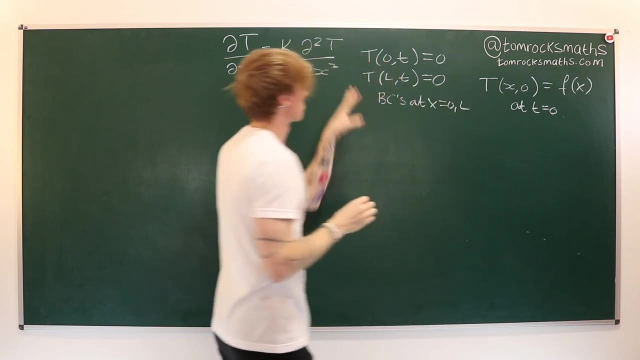 because we have an initial condition, and remember this one is at t equals zero, so the beginning state of the temperature in the rod. We have our boundary conditions, so these are at x equals naught and x equals l. and here we're going to solve it for a. 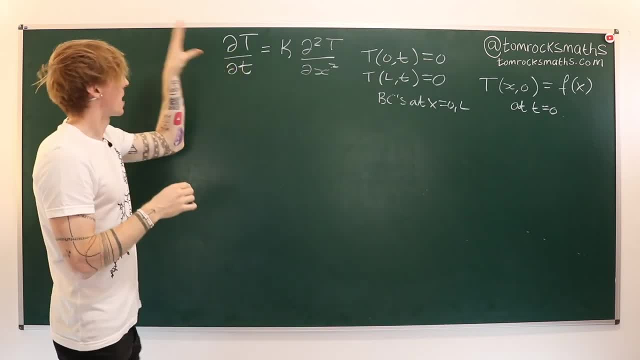 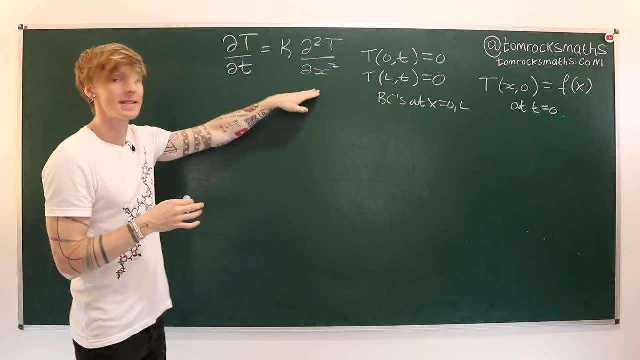 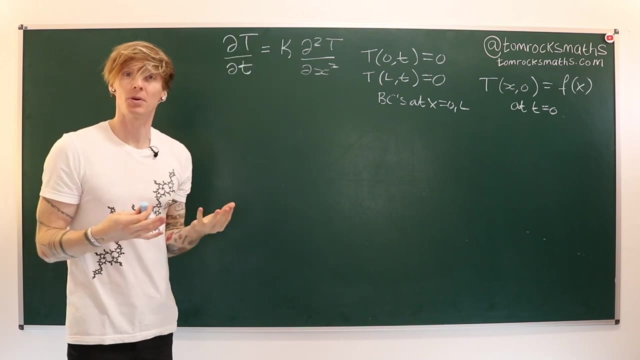 zero temperature at both end points, And then we have our actual differential equation, or pde, in two variables. The temperature will be a function of both space, x- and time, t- And this whole problem setup is, for most people, going to be the first example of a real world initial boundary. 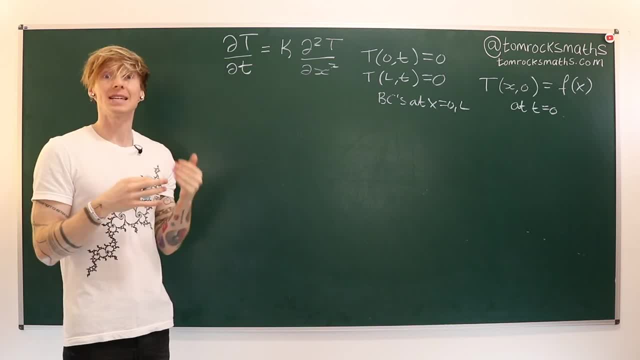 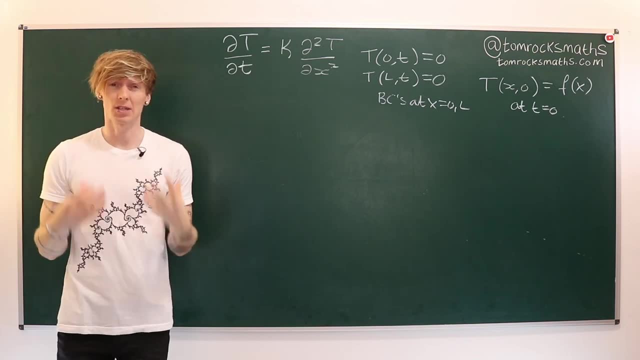 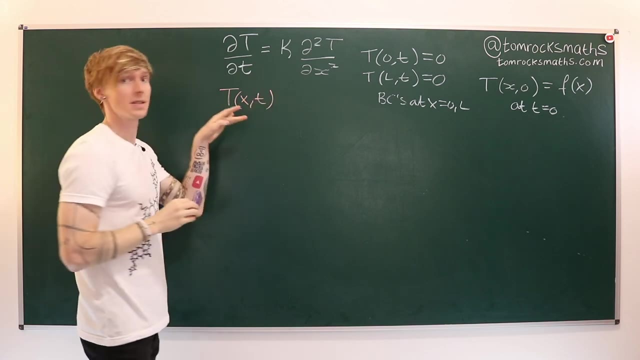 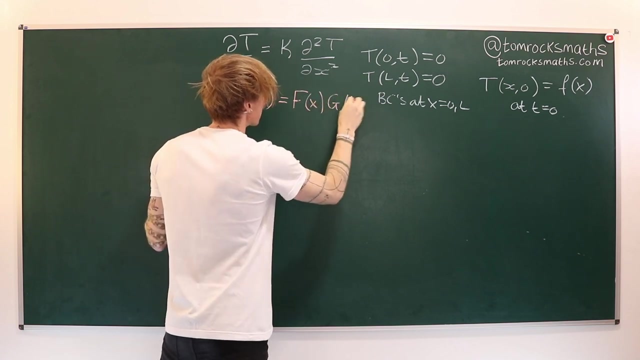 value problem. IBVP, that you will see as a maths undergrad- Our starting point is going to be to look for a so-called separable solution. So what that means here is that our temperature profile, t of space, x and time t. We're going to look for solutions of the form f of x multiplied by g of t. 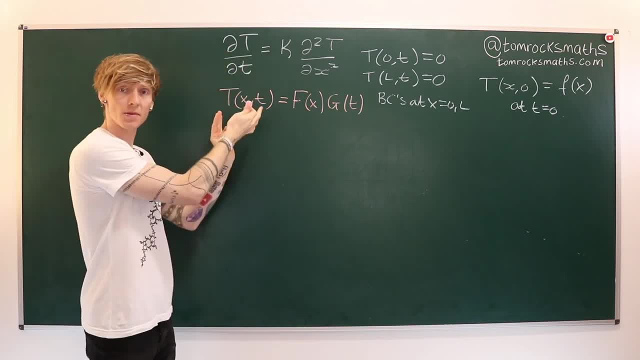 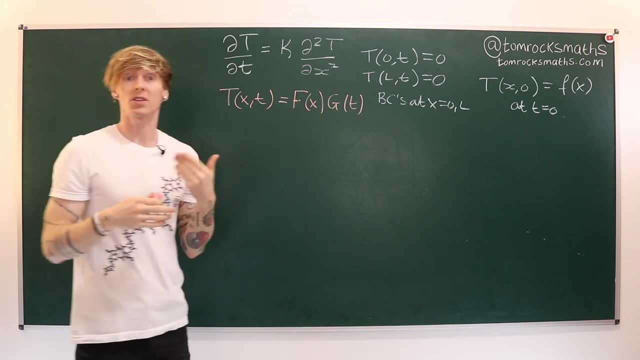 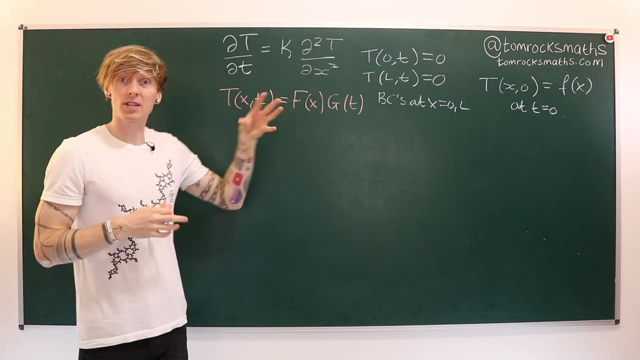 So what we've done here is separate the function of two variables into two individual functions. The first one is a function of x only and the second one a function of t, So we're going to look for a function of t only. Now I did cover this technique and how in general this works and the 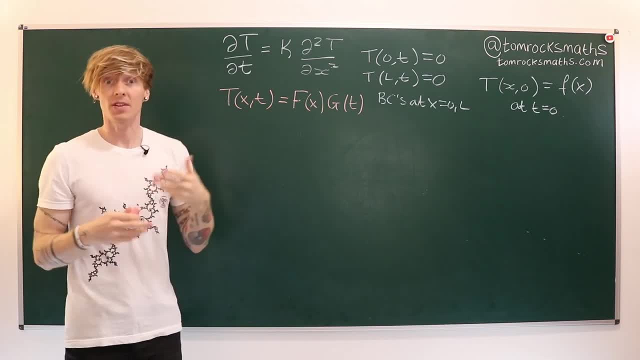 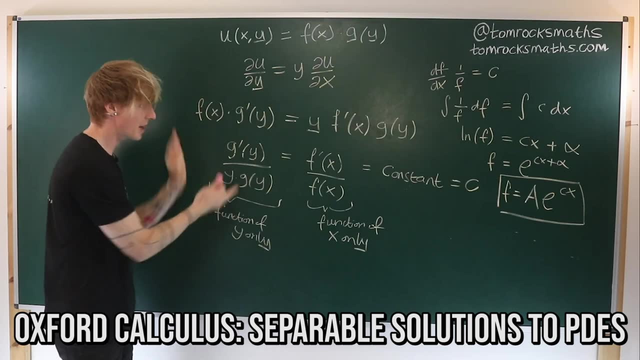 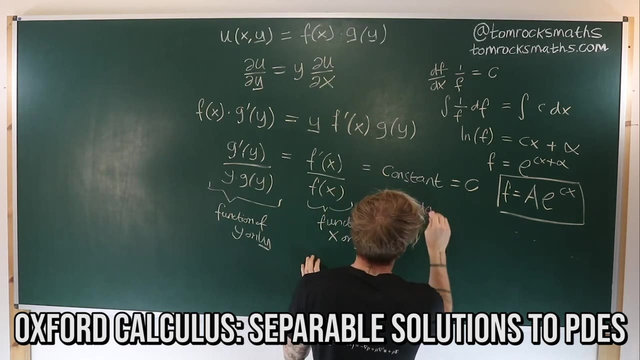 type of equations where you might try this in a previous video. So if you haven't come across this before or you've yet to watch that video, I do recommend checking that out for lots of explanation behind the method and why it works, and also some examples so you can see it in practice. 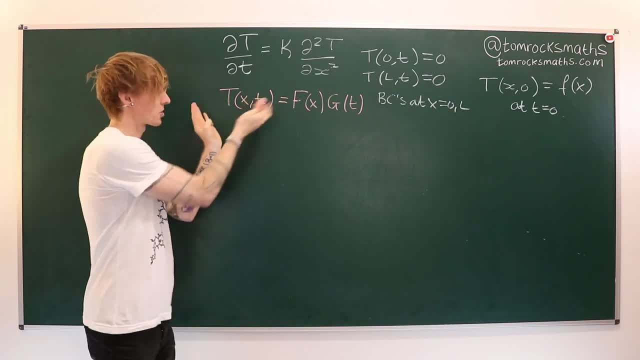 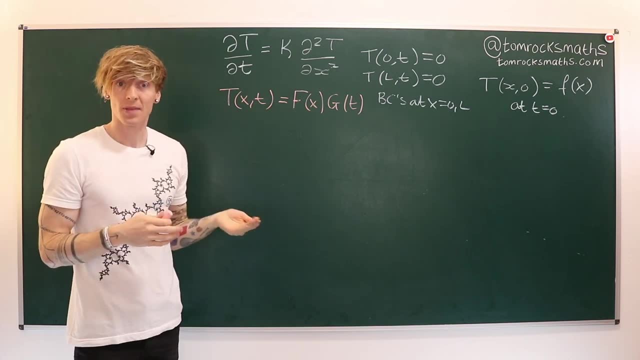 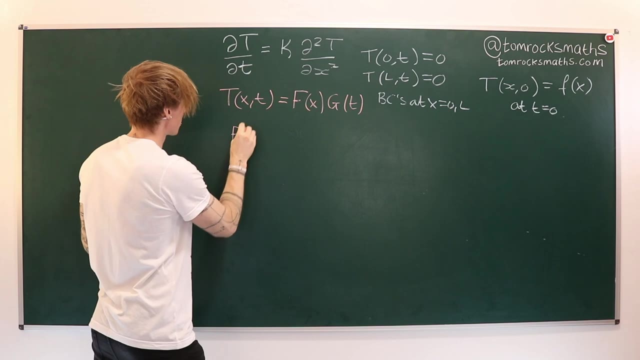 But here I'm simply going to assume that a solution of this form exists, and then what we're going to do is substitute this into our partial differential equation, So doing precisely that we're going to take a time derivative. So f is left alone, so we 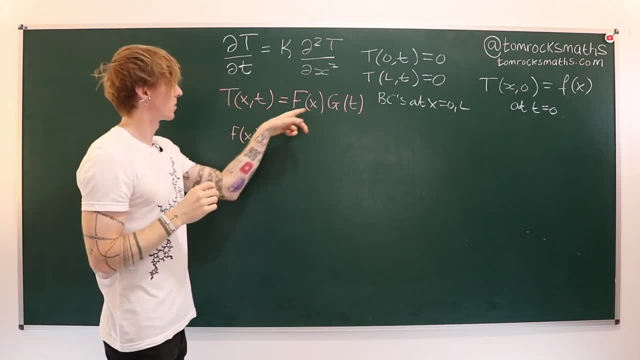 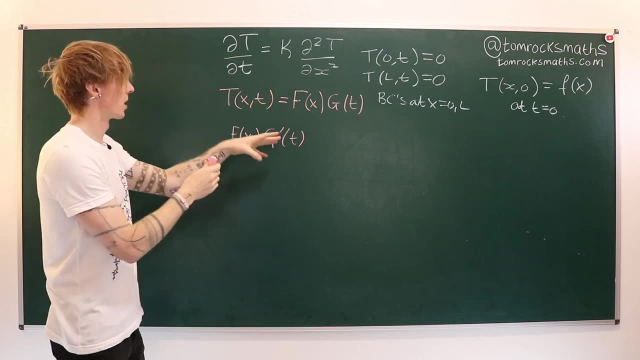 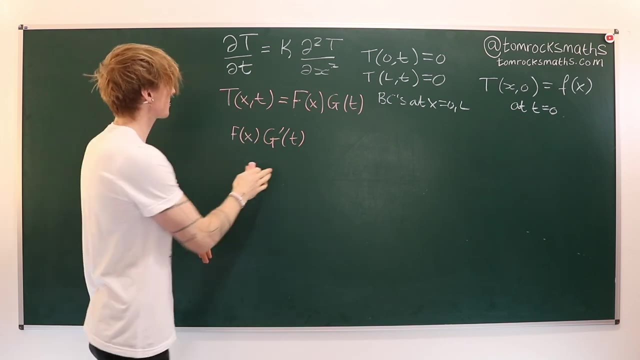 have f of x, Then taking the time derivative, we will get a g prime of t, where prime here denotes differentiation with respect to the only variable that this is a function of. So here prime has to mean time derivative. And then on the right hand side this has to equal our constant kappa times two spatial. 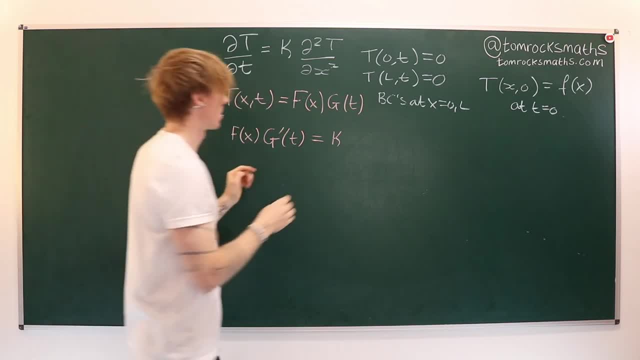 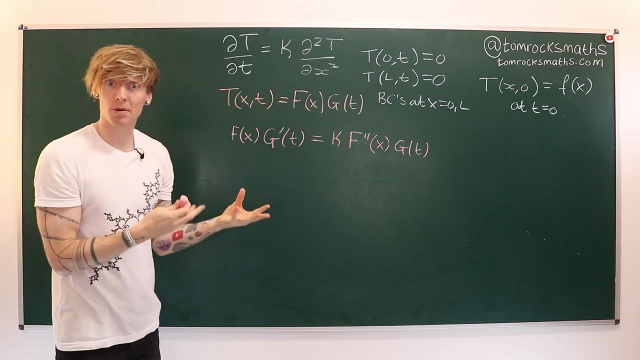 derivatives. So now we will get an f double prime of x, and the function of time g of t remains unchanged. Now what we do- and again following the general approach when looking for separable solutions- is to group together all of the terms. 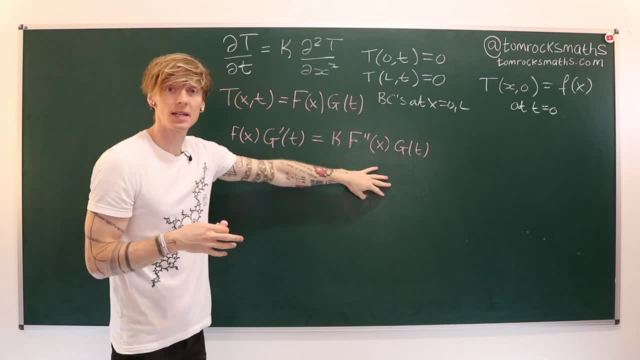 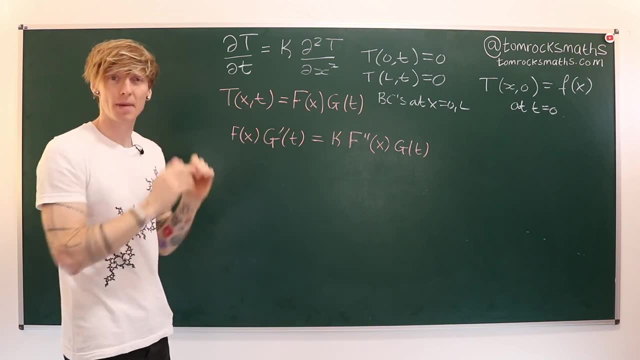 So we're going to take a time derivative. and we're going to take a time derivative and we're going to put all of the x terms on the right hand side and all the time terms on the left hand side. So if I divide through the whole equation by f times g, then what's going to happen is the left. 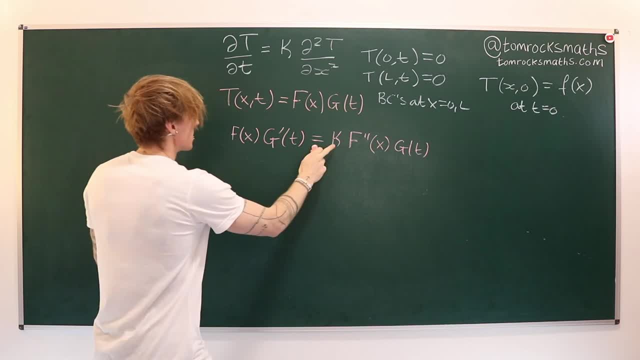 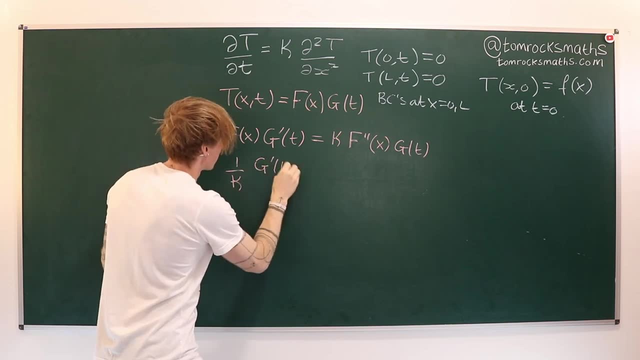 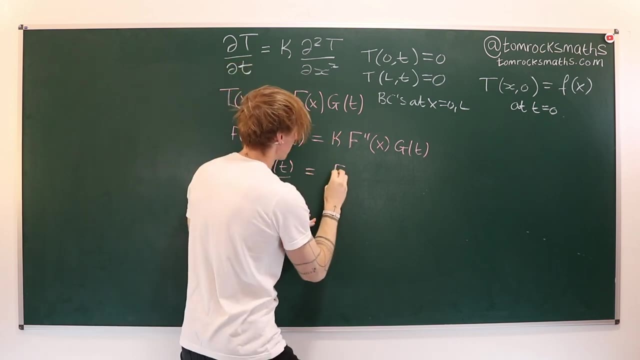 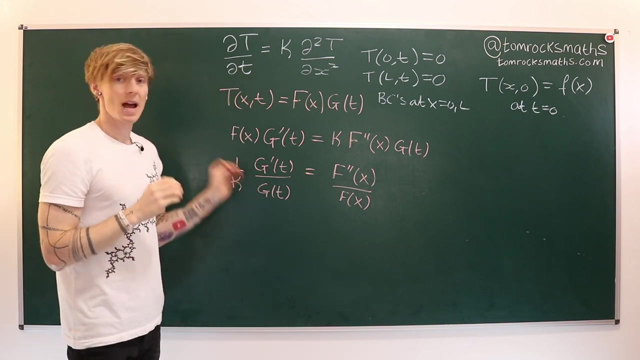 hand side and I'll also take the kappa across as well. So we take the kappa across. I'm going to get 1 over kappa. Now I'm dividing by f times g. so I have g prime of t divided by g of t, and that's equal to f double prime of x divided by f of x. Now, again following the usual method, 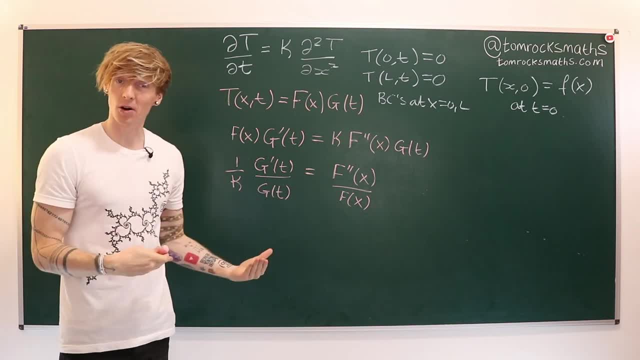 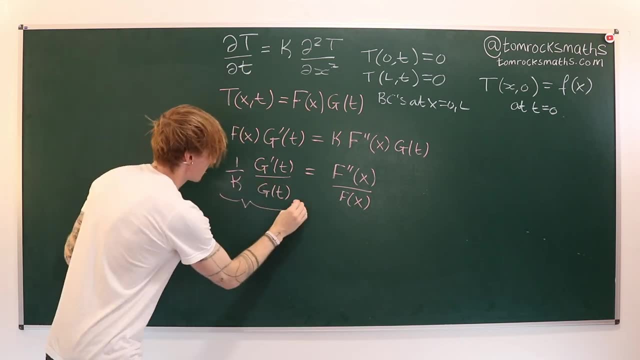 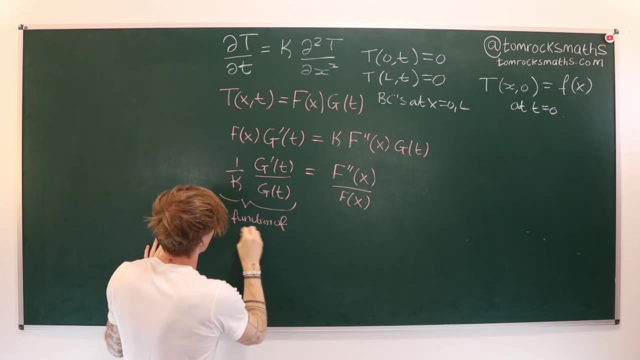 of solution. when looking for separable solutions of this form, we hopefully note that at this point, everything on the left hand side here is a function of t only, Where t here is, of course, for time, and everything on this side is a function of x only. 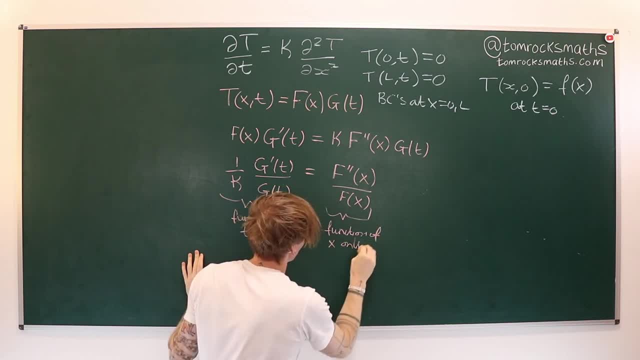 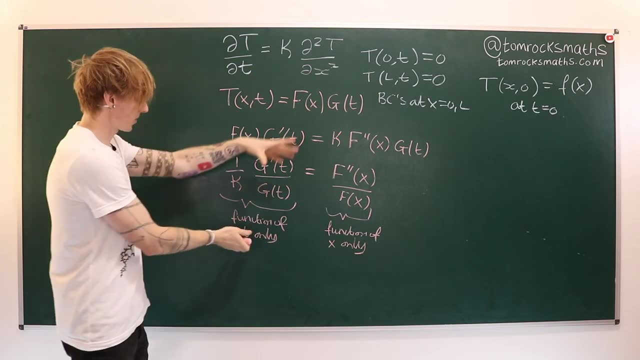 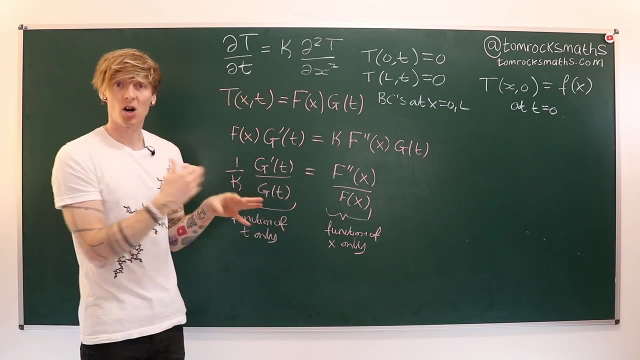 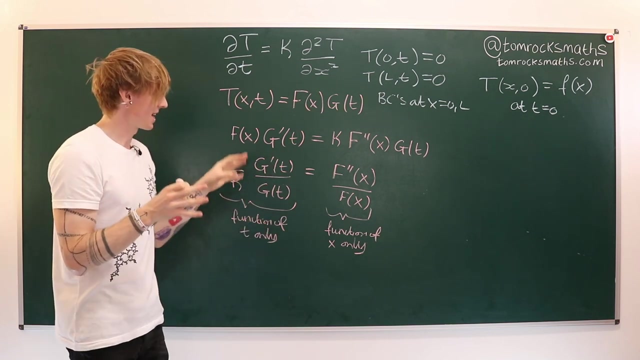 Where x here represents our spatial variable. So the only way that we can have these two things equal: we have a function that's only dependent on time, t, and another function that's only dependent on your spatial variable, x, But yet they are equal. So the only way this could happen is if both of them are equal to a constant. 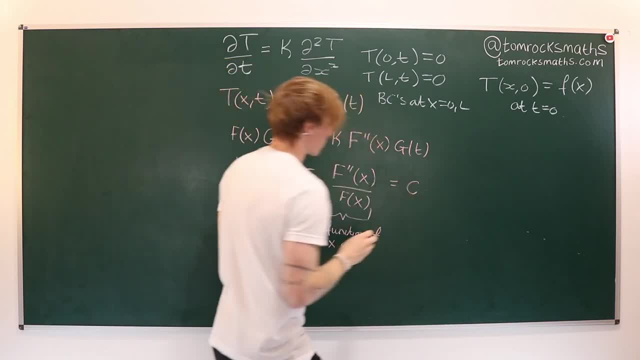 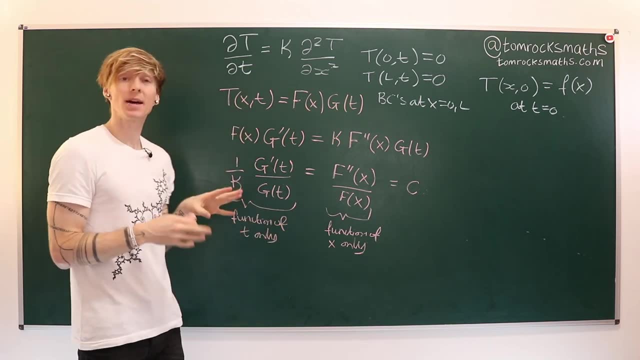 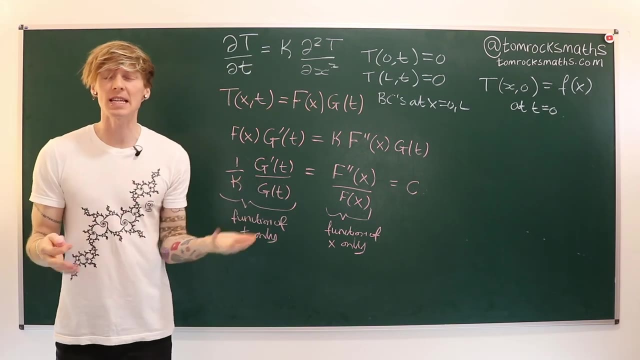 So what we're going to do is say: suppose both of them, therefore, are equal to a constant c, and now the more involved steps in this method of solution are going to be to consider the possible values which c can take. Now, this constant c can, of course, take any value, and in fact, 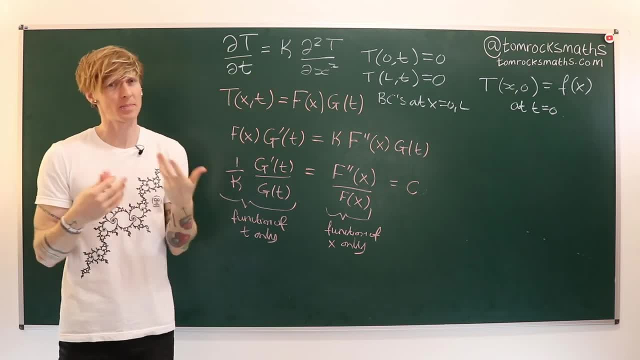 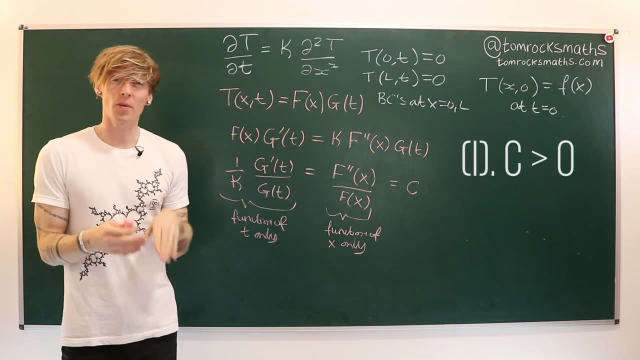 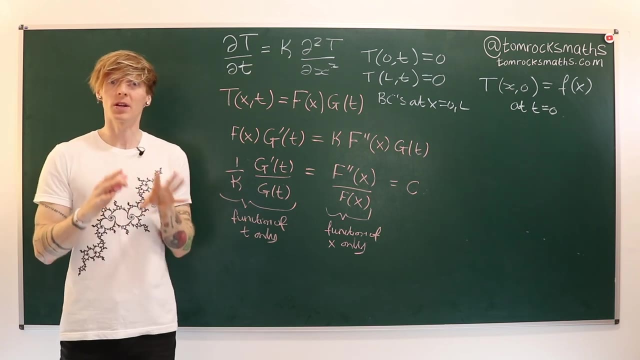 in terms of the different form of the solution which we could obtain. there are three specific cases that we need to look at, So we will consider case one, where c is positive, case two where c is zero and case three where c is negative, And what we're going to do is solve this equation. 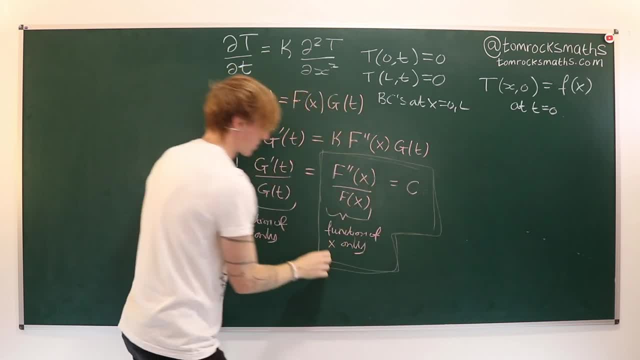 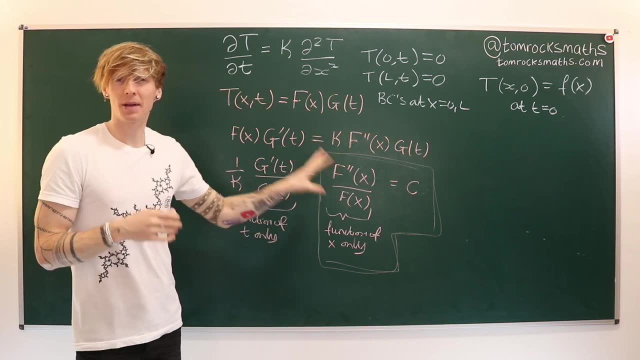 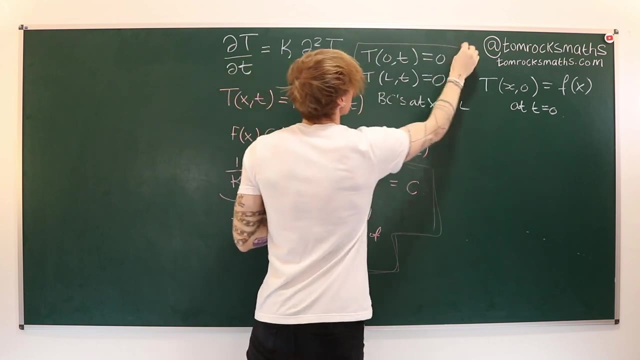 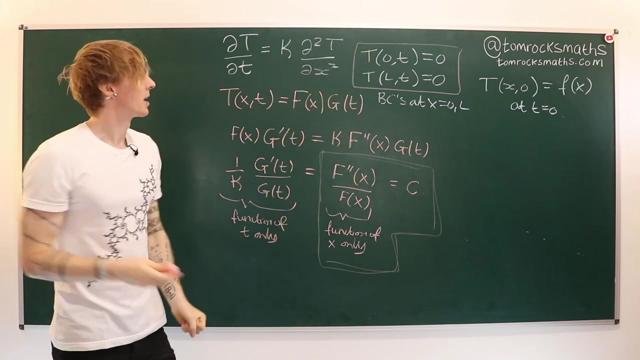 so the equation in x. we're going to solve this for those three cases of positive, negative zero. and remember we also have to apply the appropriate boundary conditions, Because up here we're told that at x equals zero, we need the temperature to be zero and 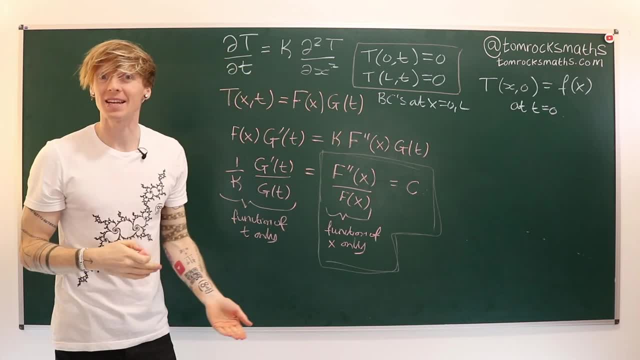 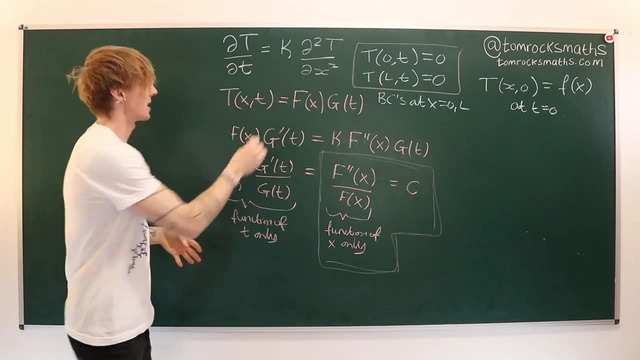 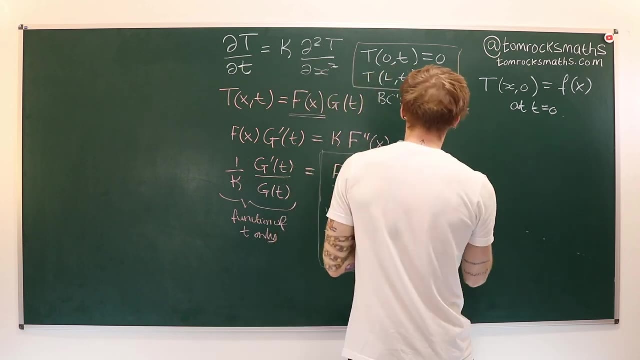 at x equals l, we also need the temperature to be zero, And because both of those are true for all time, the only thing that can be zero in our solution is actually going to be the function of x, f of x. So our boundary conditions we actually are going to solve here. 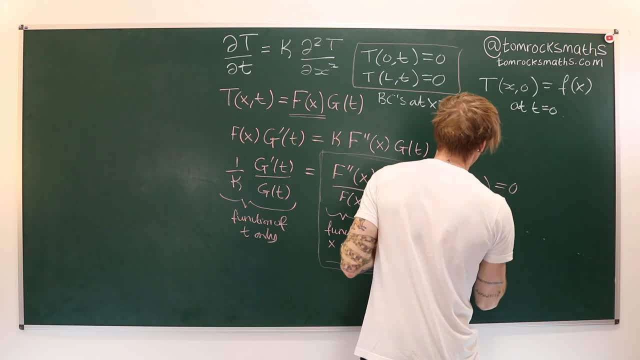 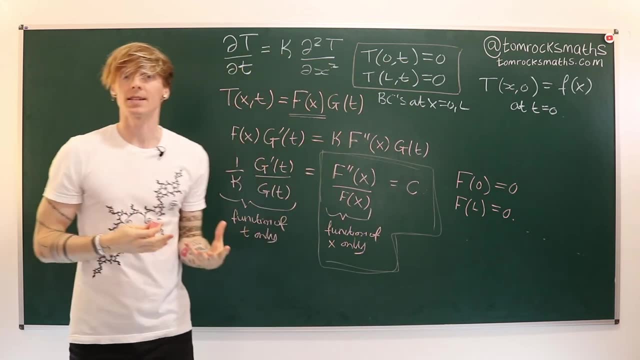 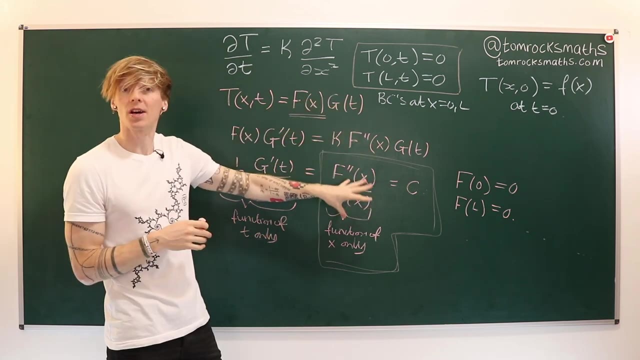 are that f has to be zero at x equals naught and f has to be zero at x equals l. So for those three cases- c positive, c being zero and c being negative- we want to solve this second order differential equation for our unknown function f and we have to apply these. 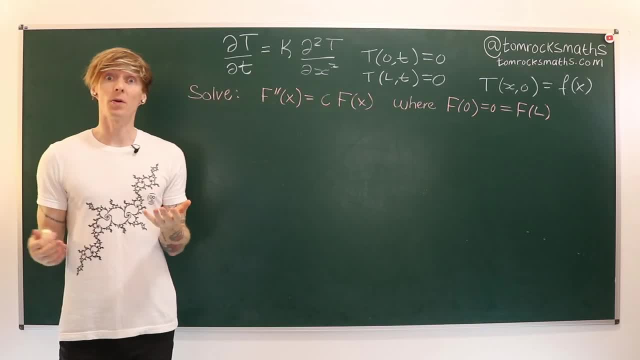 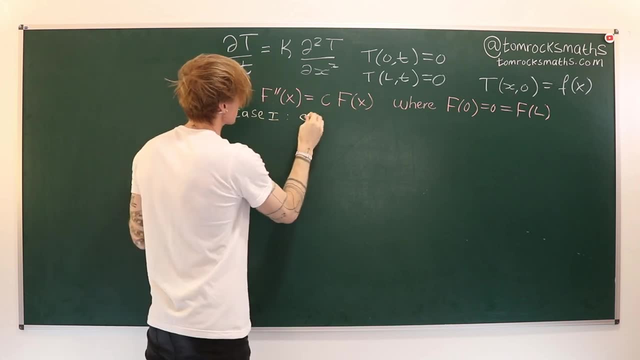 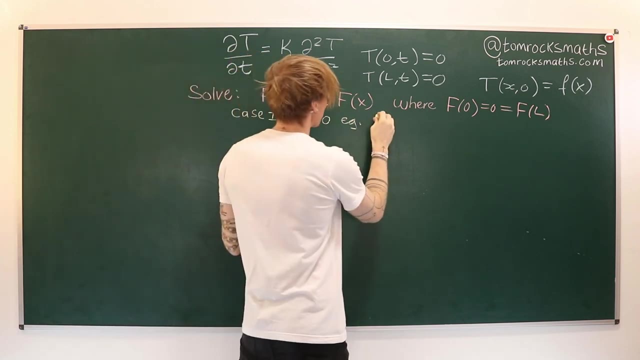 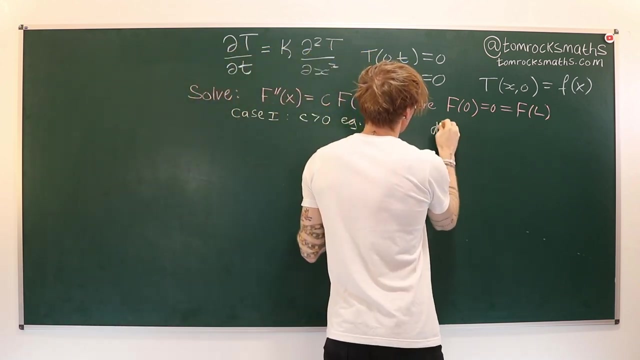 two boundary conditions. Case one will be, for c, positive. so that will mean that c is greater than zero, and I'm going to give an explicit example just to really clarify what's happening. We could, for example, take c to be one and then in this instance we would actually be solving d2. f by dx, squared is equal to. 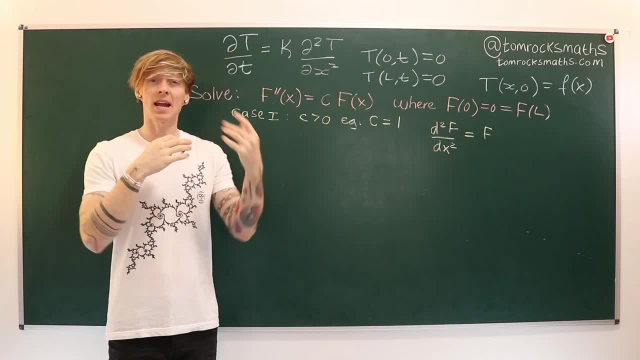 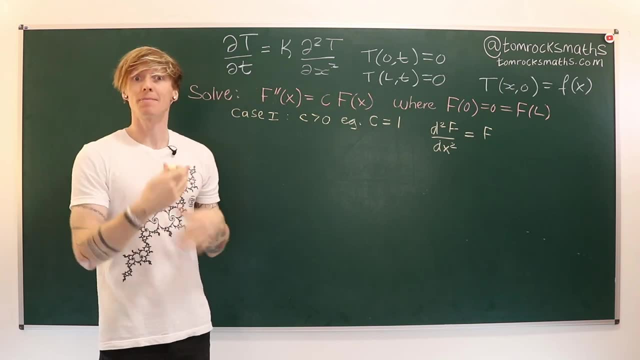 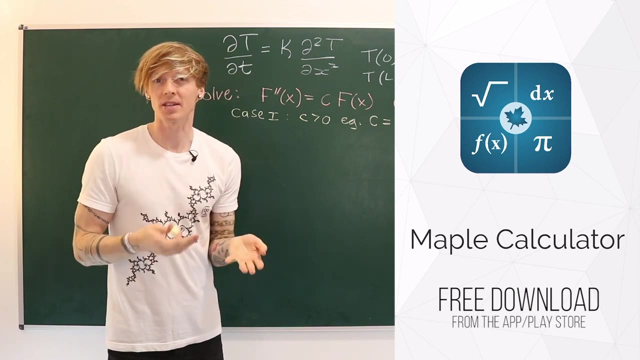 our original function f Now for each of these cases. the other reason I'm going to give an explicit example is I can actually use the Maple calculator app on my phone to solve these differential equations and then click on the steps button to see a step-by-step breakdown of how the 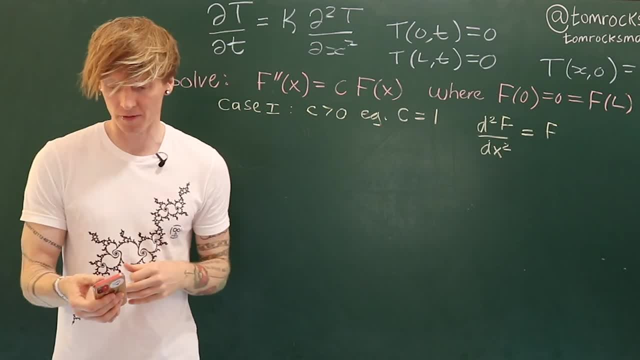 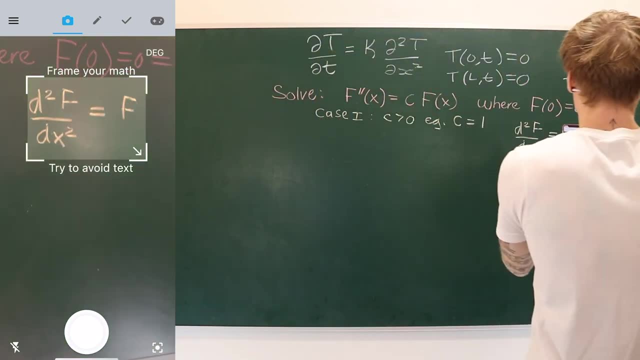 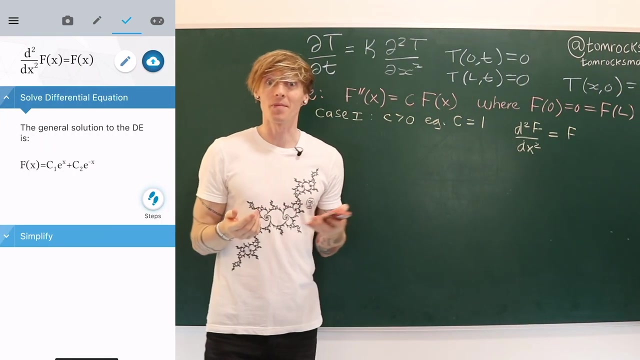 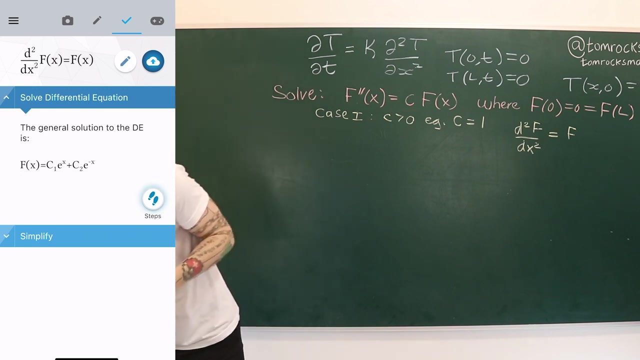 solution was found. So if I open the app on my phone, then I can click on the camera tool at the top of the screen. I can actually just take a photo of the equation that I'm trying to solve and then this appears now on my phone and it tells me the general solution to this differential equation, which is given. 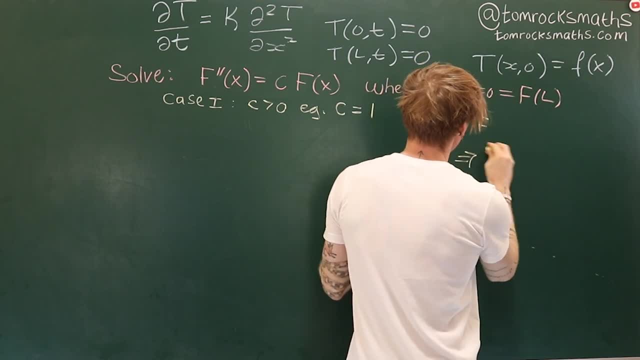 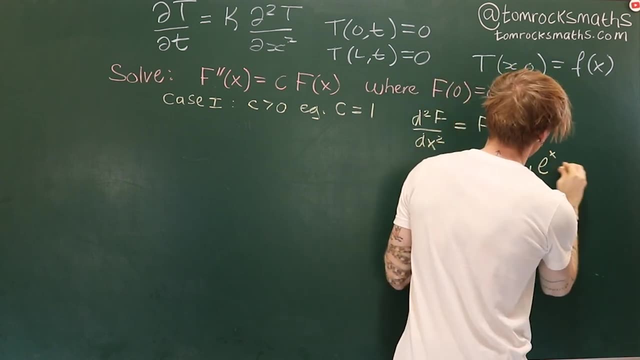 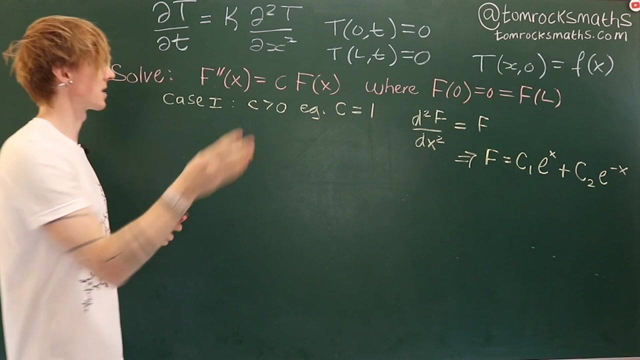 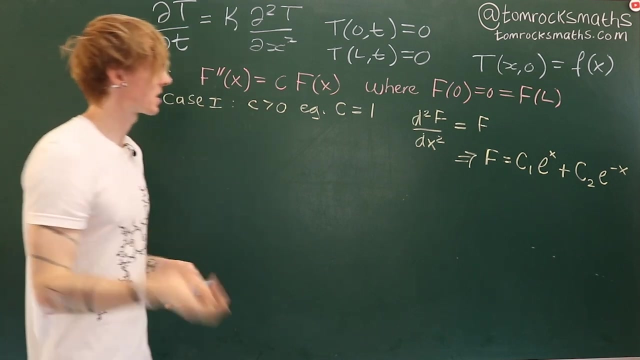 by f of x is equal to c1, e to the x plus c2 minus x. Now remember, this is in the specific case when c is one. the solution is very similar. if I have a positive c, all that will change there is I will have a square root of c. 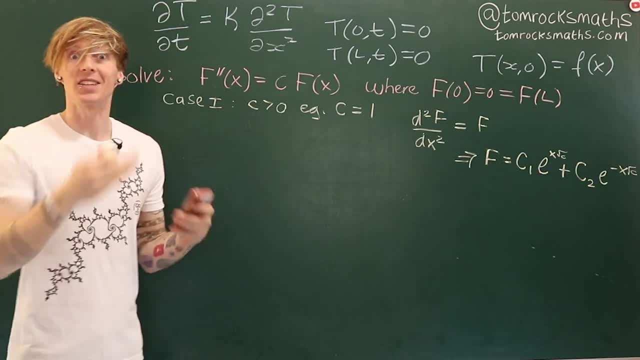 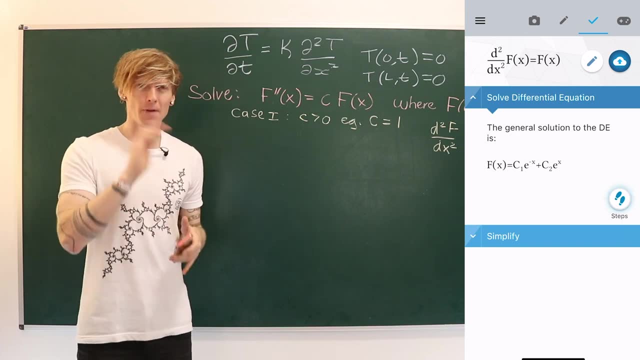 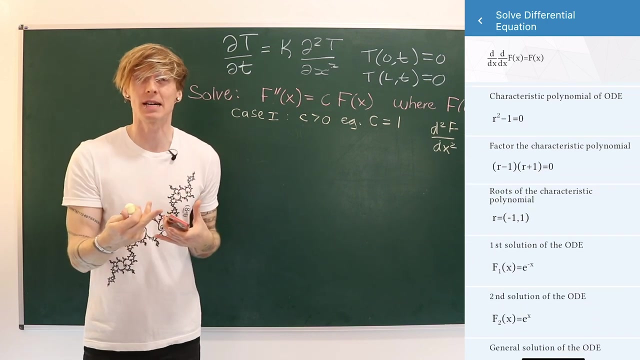 at the top of both of those exponential indices And remember. if you're unsure as to where this solution has come from, then you can always just click on the footprints icon, the steps button, on the Maple calculator app, And it will give you a step-by-step breakdown of how the solution was derived. 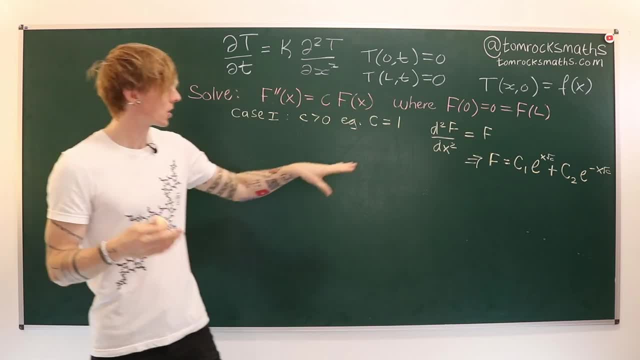 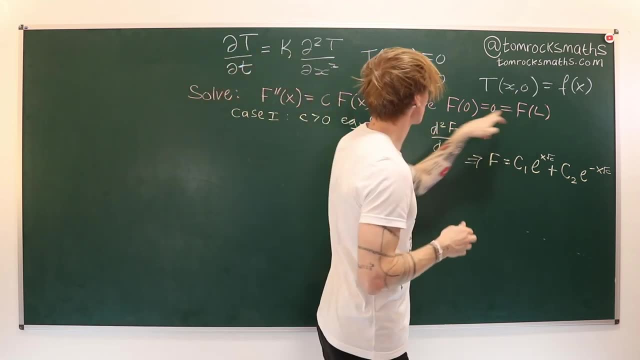 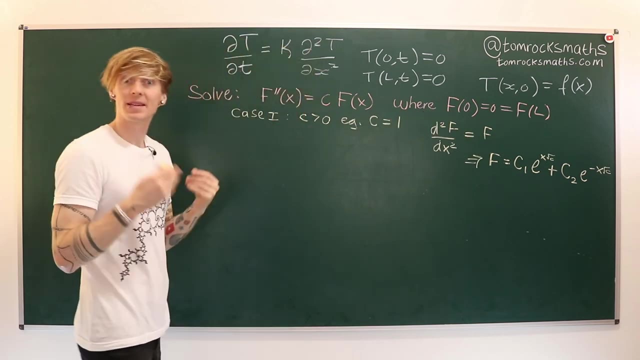 At the moment we have the general solution for our unknown constants c1 and c2, but recall that we actually have a boundary condition or two boundary conditions that we need to satisfy. So if we apply f of 0 must be 0, then that's going to tell us that 0 must equal. 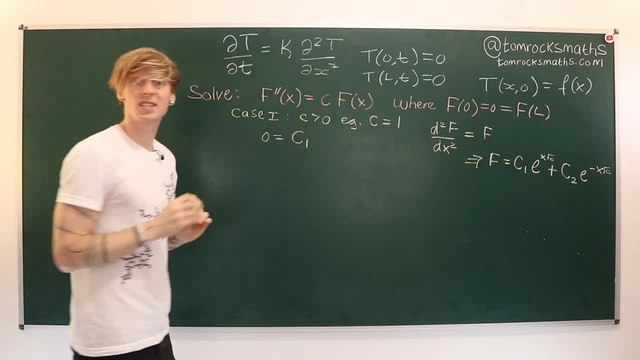 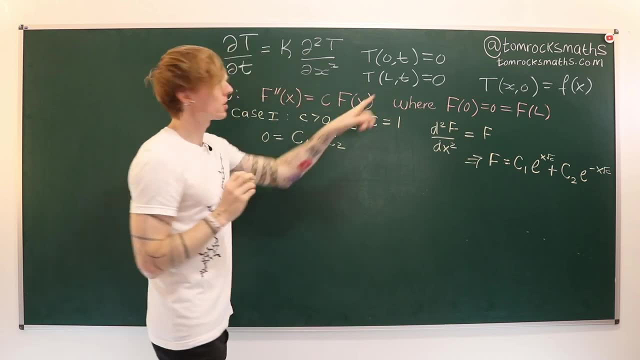 c1, e to the x plus c2.. times e to the 0, so that's just c1 plus c2. times e to the 0, so that's plus c2. and then we also need f of l to be equal to 0, so that's going to tell us. 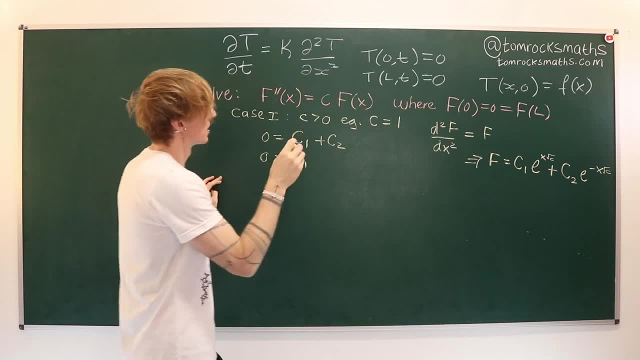 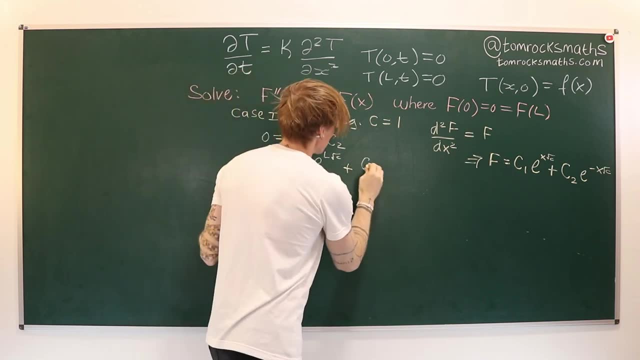 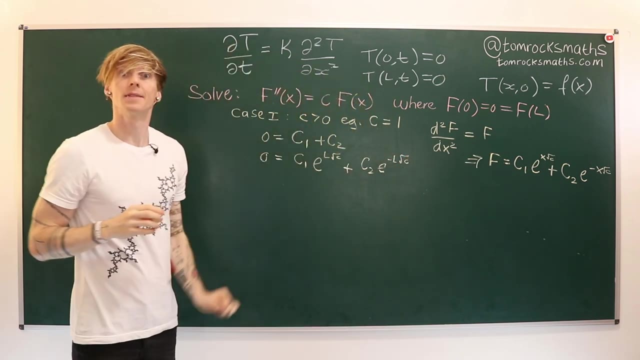 that 0 has to be equal to c1 times e, to the l times the square root of c, plus c2 times e to the minus l times the square root of c. Now we have a pair of equations, two equations in two unknowns: c1 and c2.. 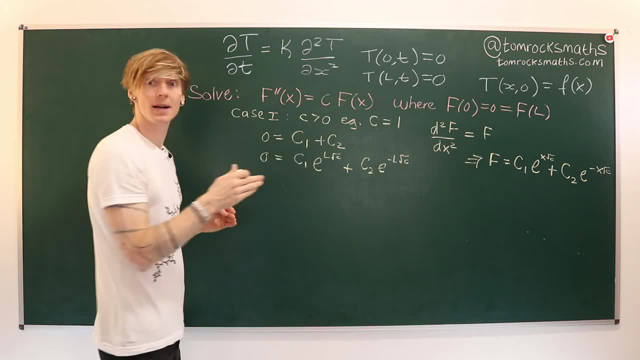 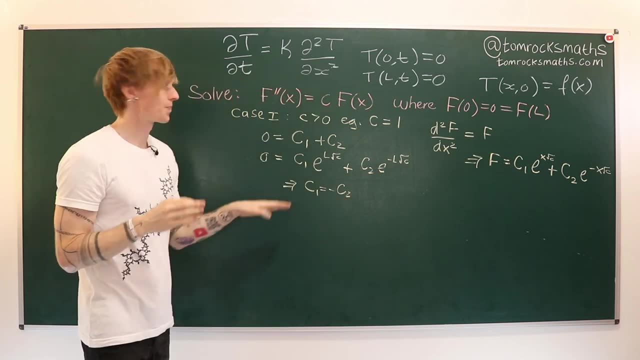 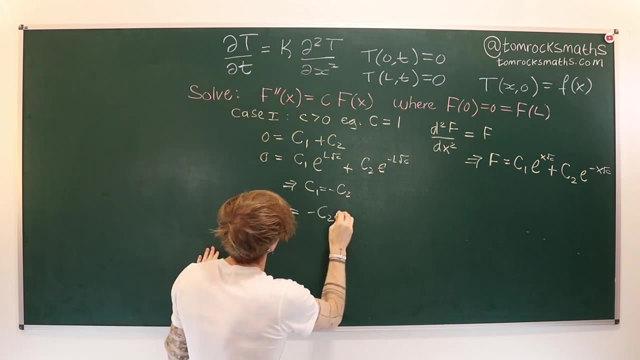 So from the first equation we can see that c1 has to be minus c2. so that tells us that c1 equals minus c2. and then if we plug that into the second equation we get: 0 is equal to minus c2. e to the l times the square root of c. 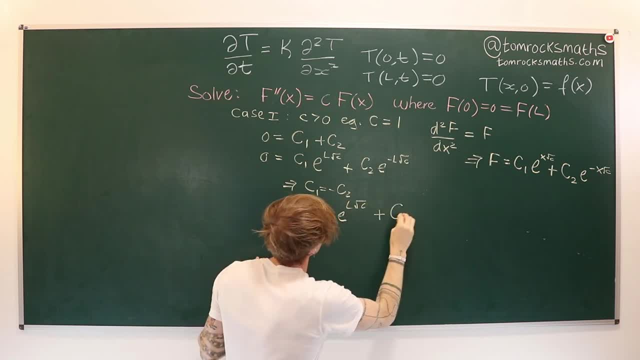 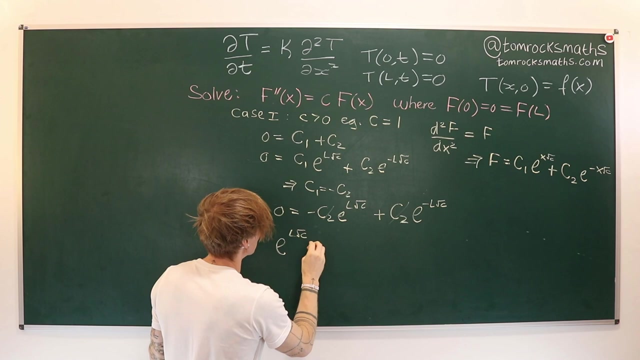 And then we've got plus c2 times e to the minus l the square root of c. So if I take this equation over and then I can actually cancel c2, what you're going to see is that this equation is only satisfied precisely when e to the l square root of c equals e to the minus l square root of c. 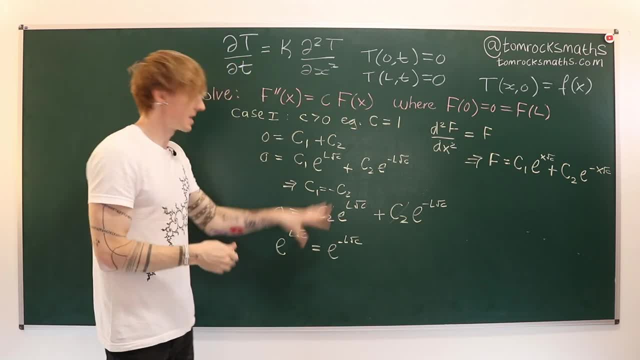 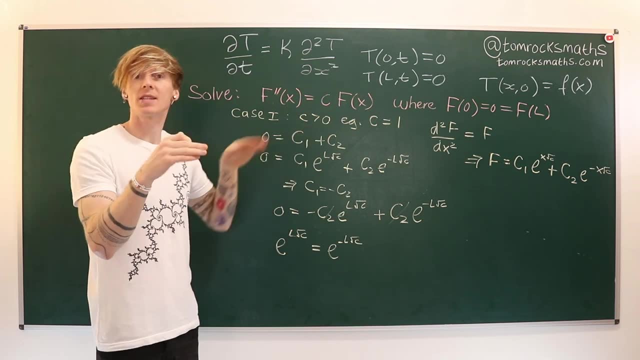 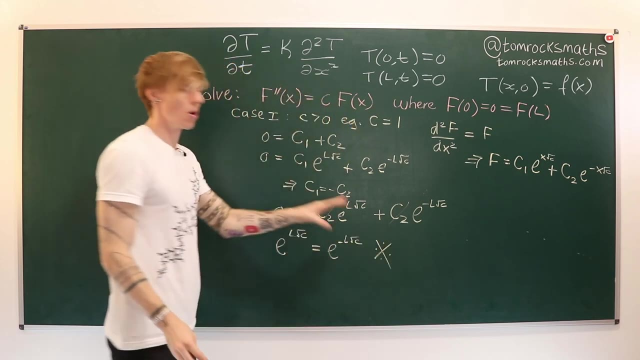 Now for a fixed value of c. this isn't going to be true, because we have said that c is strictly positive. It can't be zero because that's going to be case two. So this actually cannot be satisfied. The only way this equation works, the only thing that makes this work, 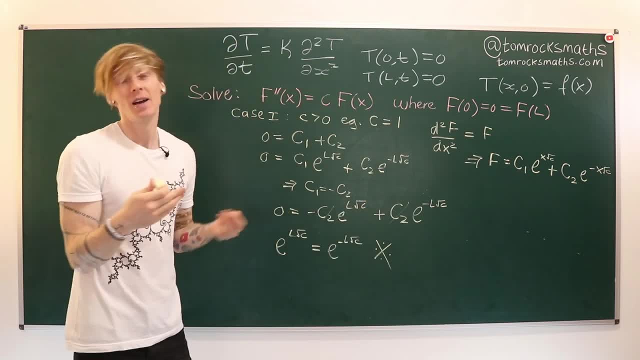 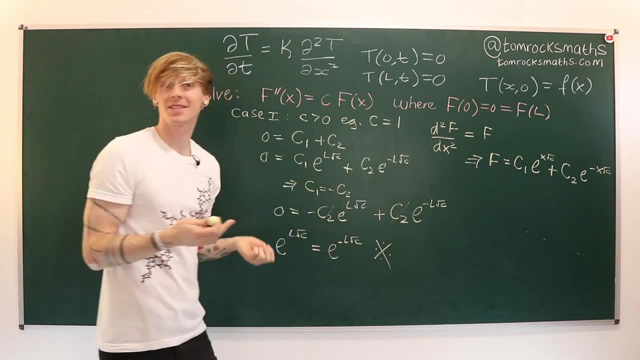 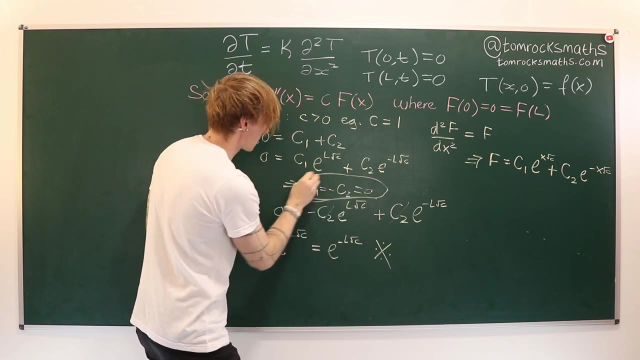 is up here. When I cancelled the c2, I had implicitly assumed that c2 was zero. If c2 is zero, of course I can't cancel them, but if c2 is zero, then c1 is zero. So the only thing that works here, the only way we can satisfy the boundary condition of being 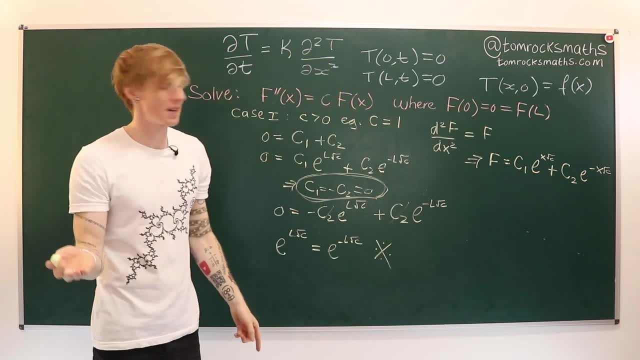 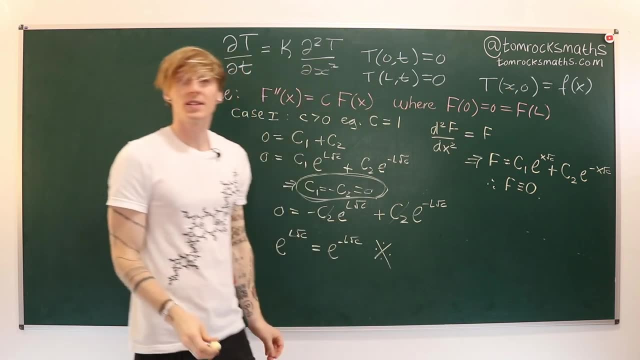 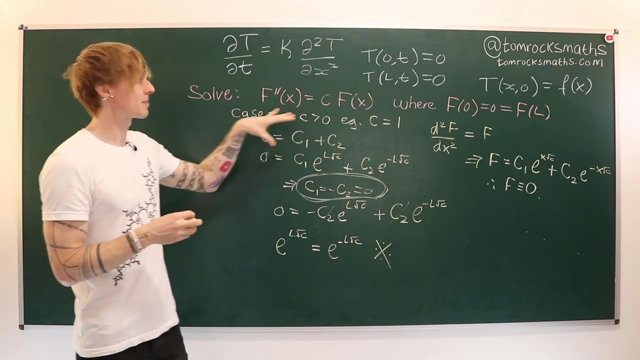 zero at the two endpoints is actually if both constants are zero and therefore our whole solution f is identically zero, which is very boring. We call this the trivial solution. So in summary, we've seen that if c is positive, case one for positive c. we've found that the only way to 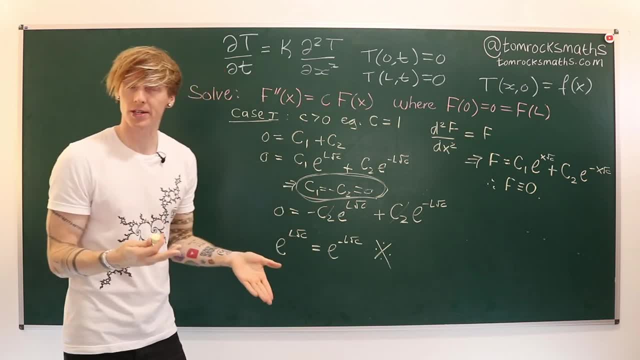 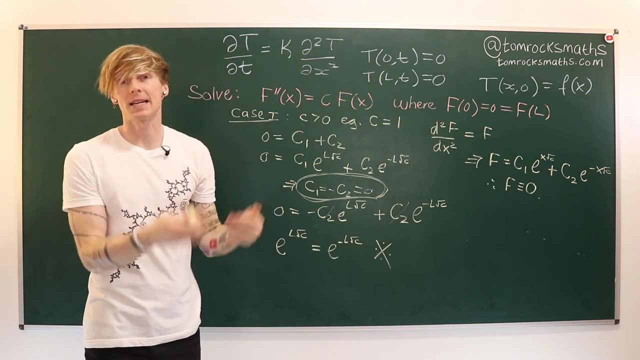 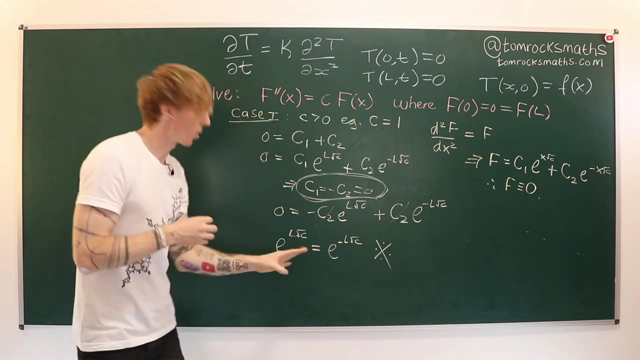 satisfy the original partial differential equation and the boundary conditions- x equals naught and x equals l- is for the solution to be identically zero. We don't care about this, it's too boring, it's trivial. So what this means is that the case one of c being positive, 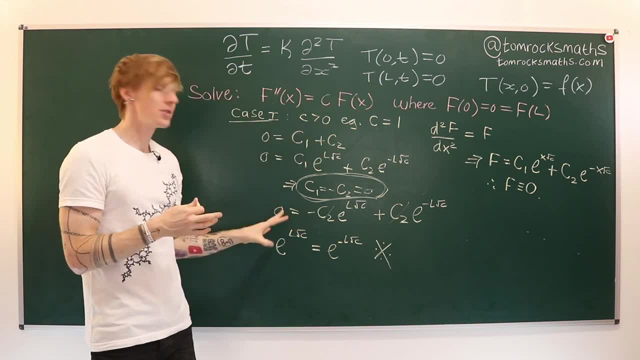 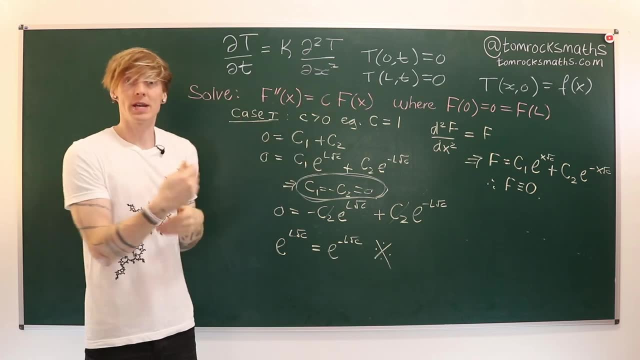 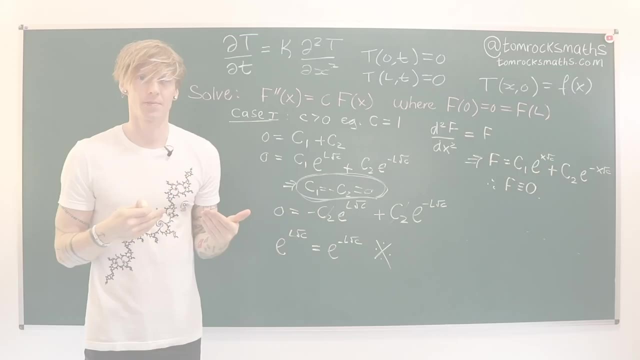 we can sort of neglect that We're aware of what happens. we've convinced ourselves it would be the boring case for this particular problem. so therefore we can go on and consider cases two and three and see if it's possible to get a non-zero solution. Case two was when c was equal. 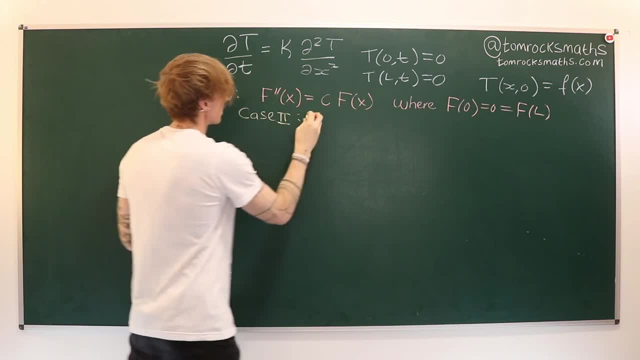 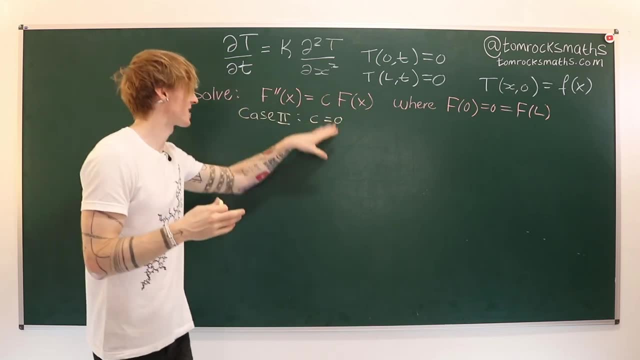 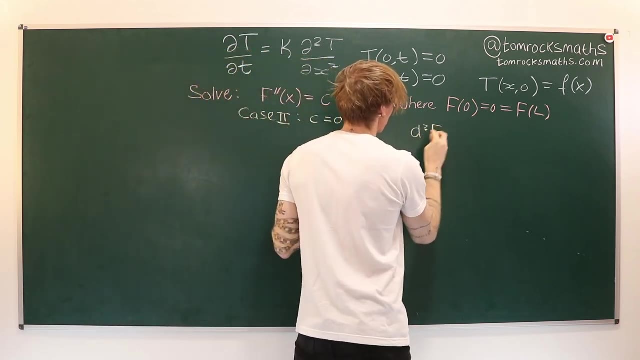 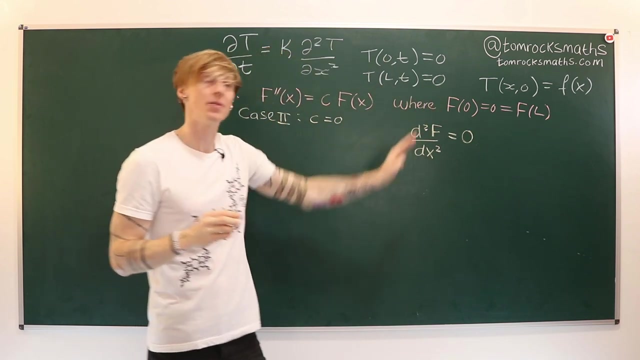 to zero. So case two, c, equals naught. Now I don't need to do an explicit, concrete example, because we have a single fixed value for c. So what we're trying to solve here is going to be: d2. f by dx squared is equal to zero, with our boundary conditions the same as before. 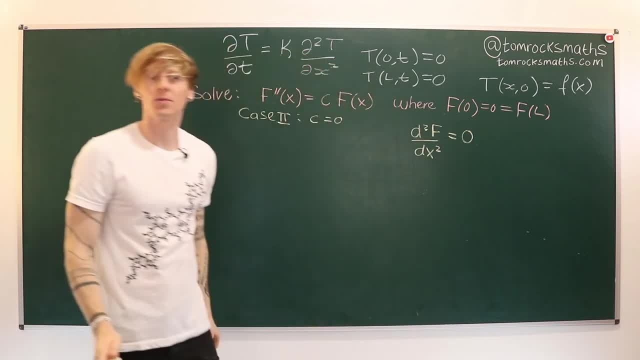 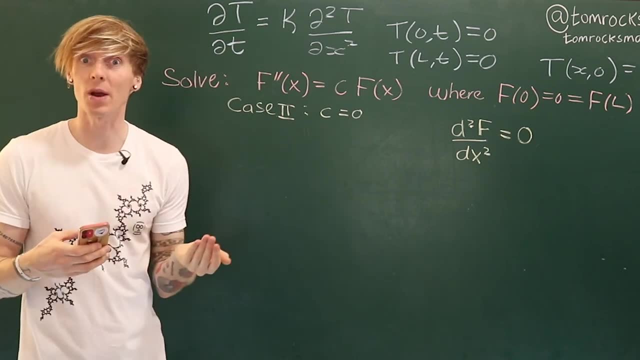 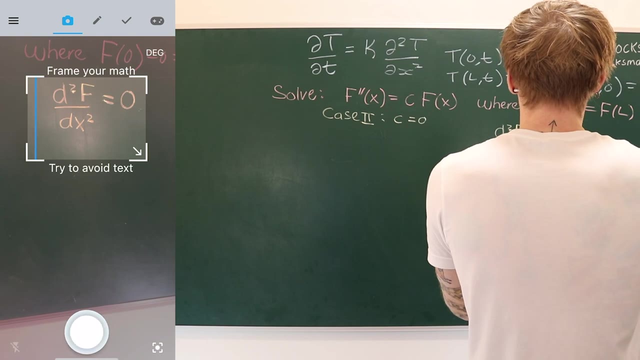 We need f of naught to be naught and f of l to also be zero. Once again, I'm going to use the Maple Calculator app to help me solve this differential equation. So if I open up the app, then I can take a photo of the new equation that I would like to solve and, as before, this will open. 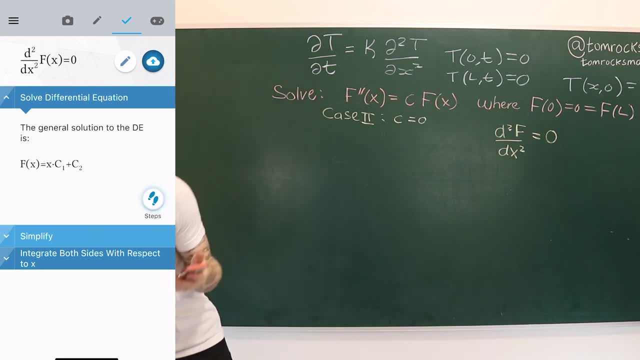 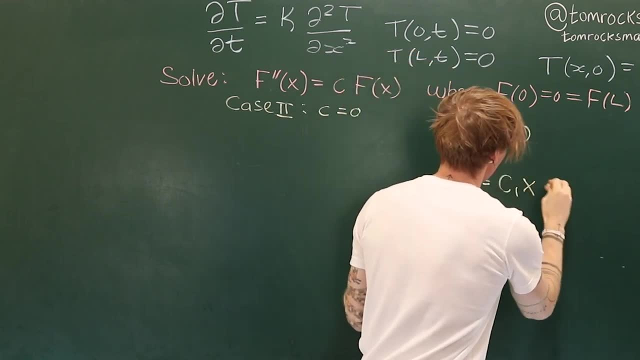 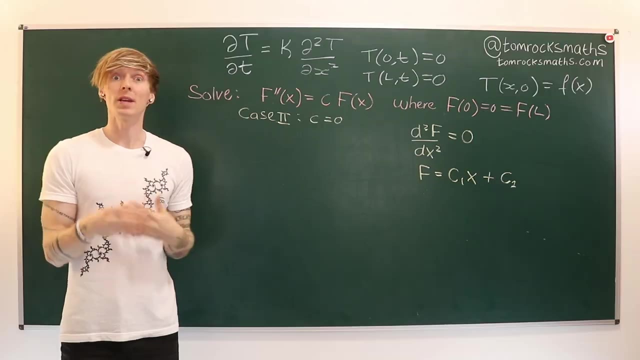 up in the app and I can now see that the solution here is given by f is equal to c1 times x plus c2.. So in this case it is a simple linear function. We continue as before and we want to apply our boundary conditions. 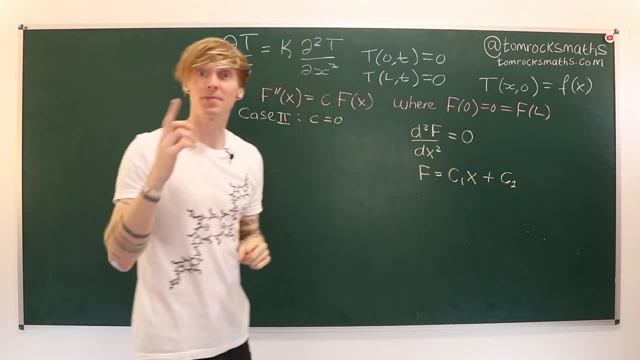 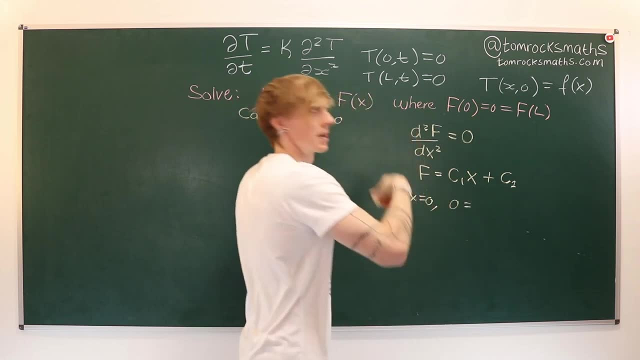 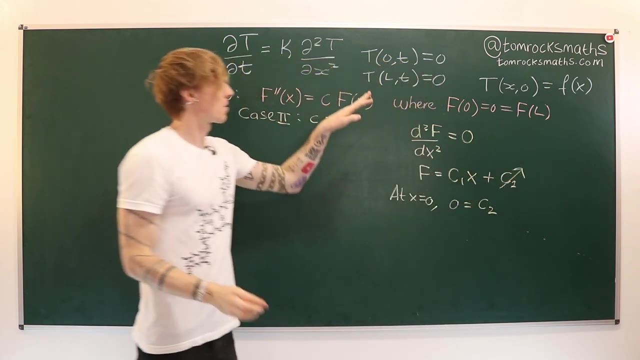 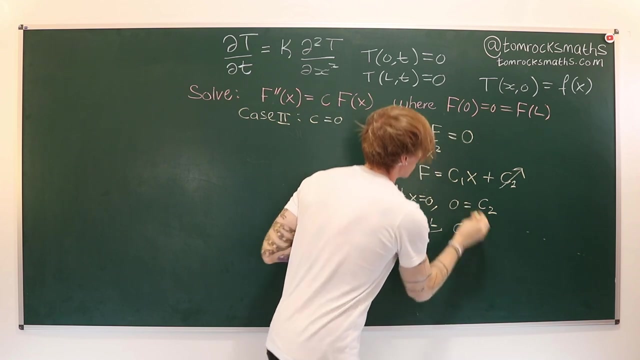 So we need: when x is naught, we need f to be zero. So that tells us that at x equals naught, we need zero equals x is naught, so c1 disappears, so zero equals c2.. So that tells us that one disappears. and then when x is equal to l, so at x equals l, we need zero is equal to c1 times l. 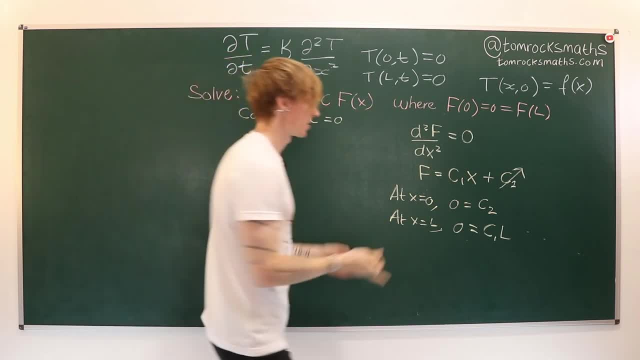 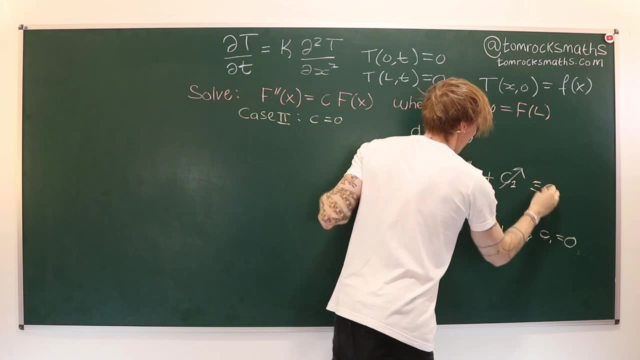 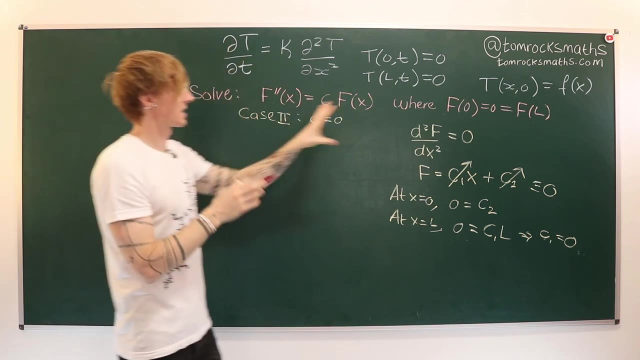 l is a non-zero Length, so that can't be zero, so we must have that. c1 is also zero, so that's zero. so f once again, unfortunately, has got to be identically zero, such that it satisfies our differential equation and these two periodic boundary conditions. 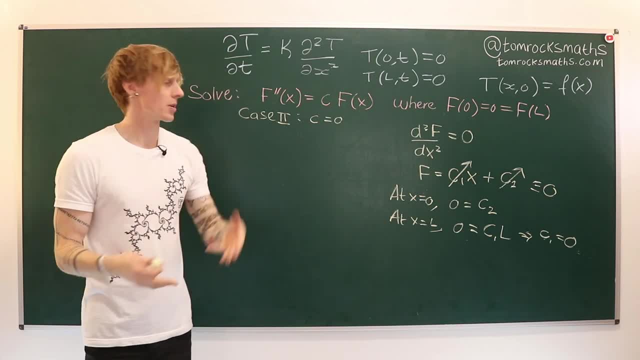 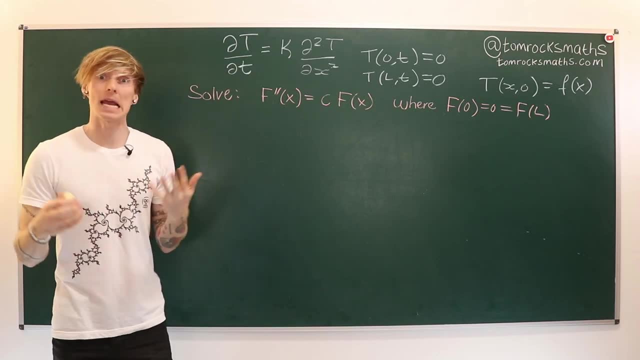 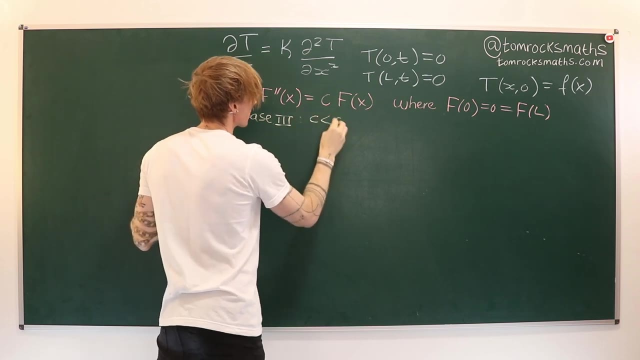 So again, this is a trivial solution, it's a boring solution. we're not interested in this, which means want to move on to case three. Our third and final case was for C negative. So case three is going to be C less than zero. and again, let's take a concrete 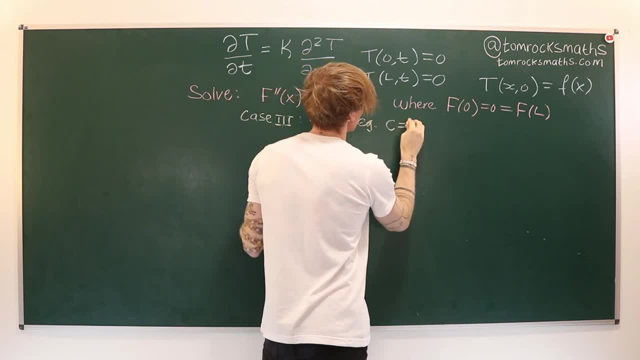 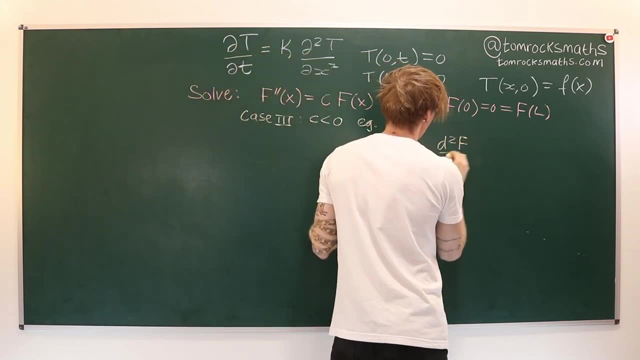 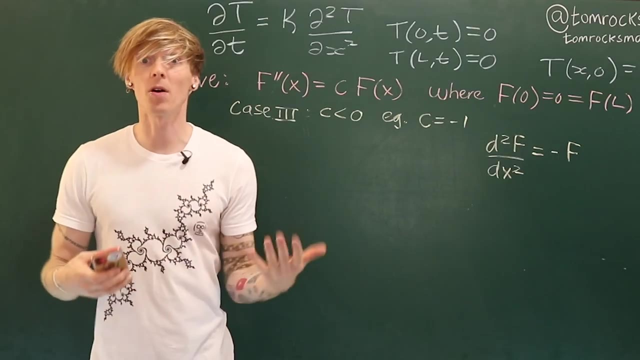 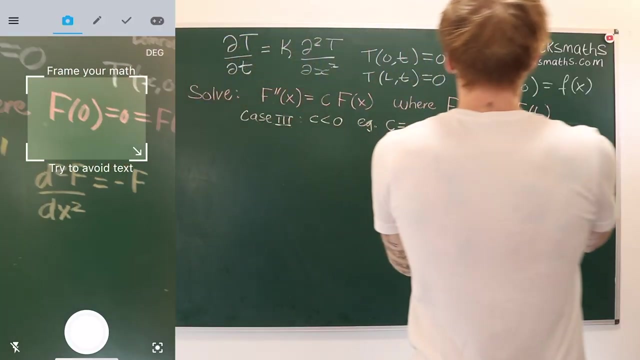 example, eg C is equal to minus one, and in that case we would be solving d2 f by dx. squared has to be equal to minus f. Just as before, I can use the Maple Calculator app to help me solve this differential equation, So taking another. 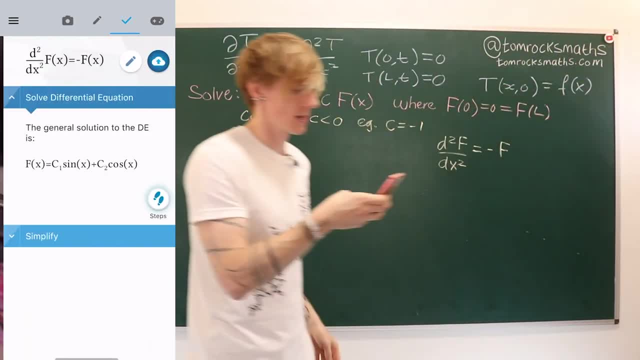 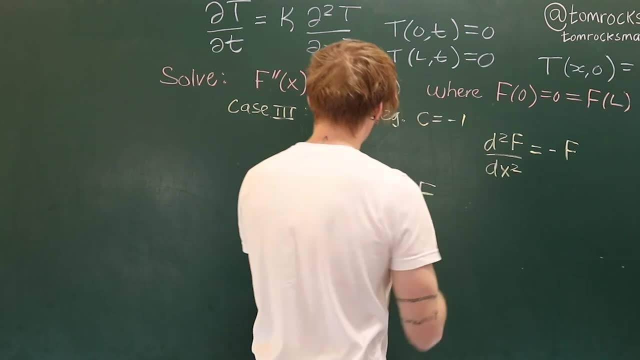 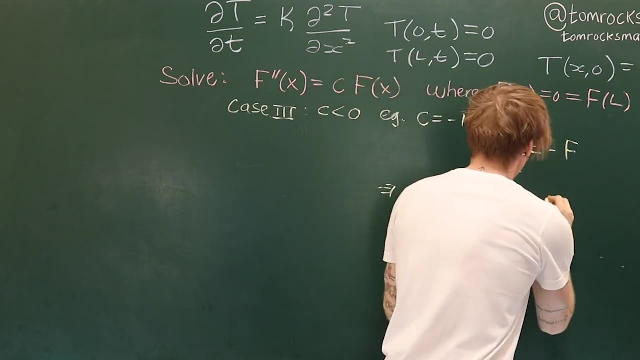 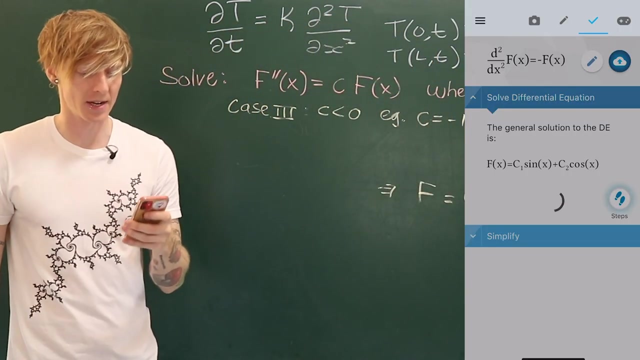 photo. this will now appear in the app and I can see that the solution in this situation is: f is equal to C1 times sine of x plus C2 times cos of x, and again I can click on that steps button and see a. 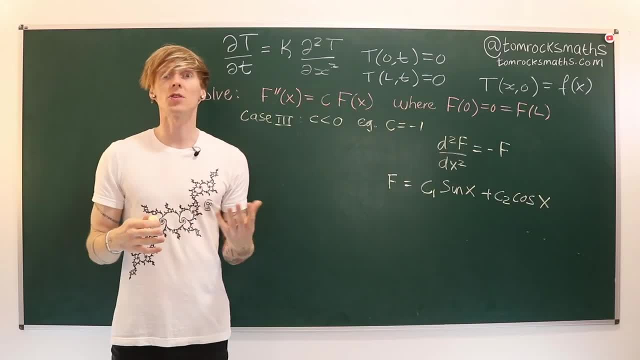 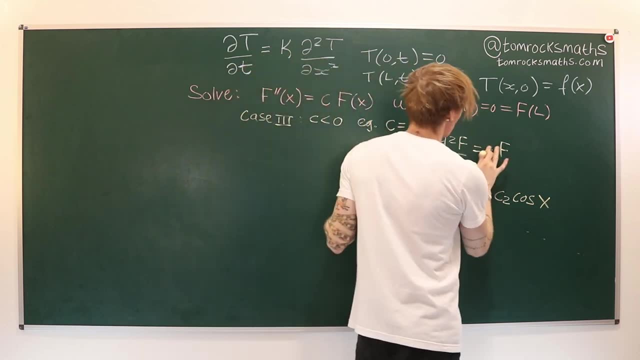 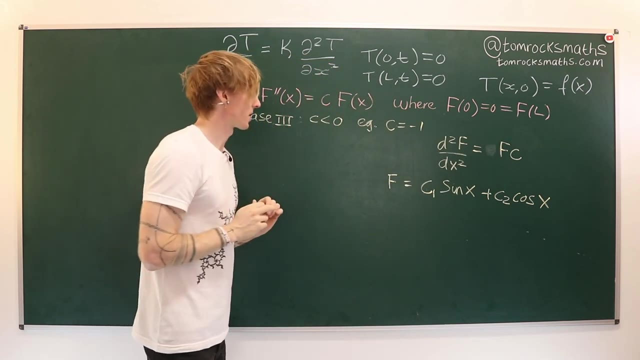 breakdown of where the solution came from. Now, this is, of course, the specific solution for C being equal to minus one. So if, instead, we replace the minus one by a generic C where- remember- C is negative, then what we're going to see here is the general solution. 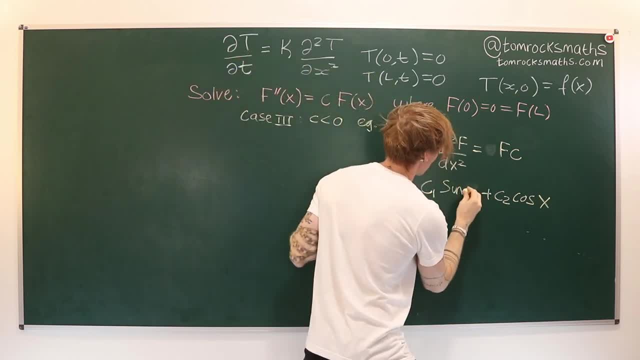 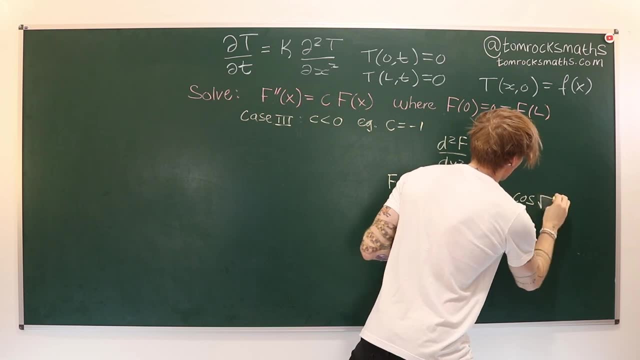 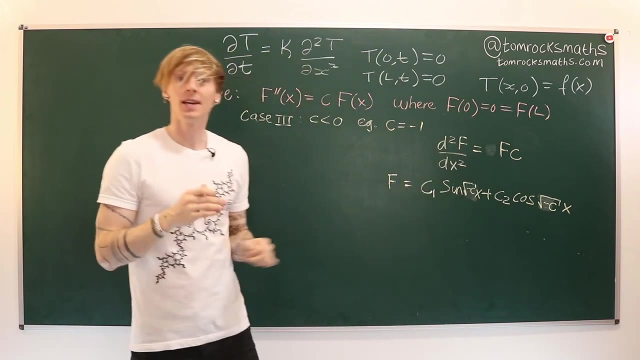 Instead of being sine of x, this is now sine of root minus C times x and similarly it's cos of the square root of minus C times x. And note the negative sign in front of C means we have a positive thing which we can square root. 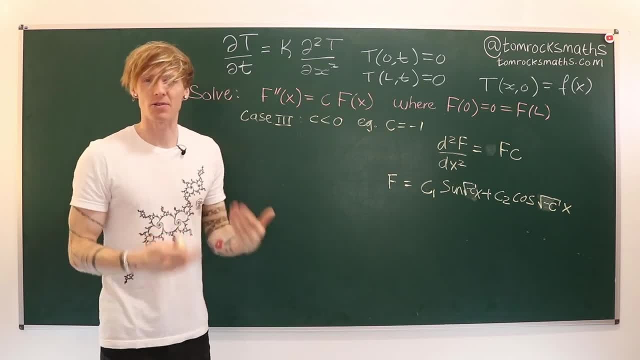 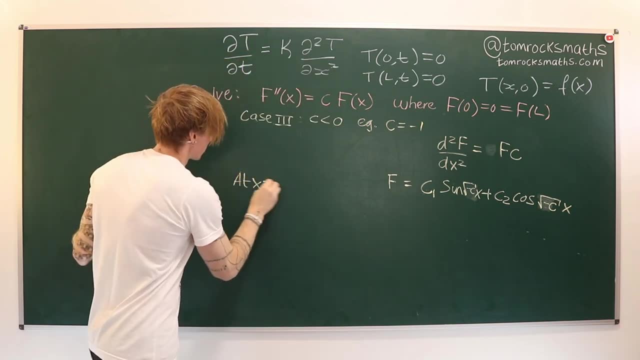 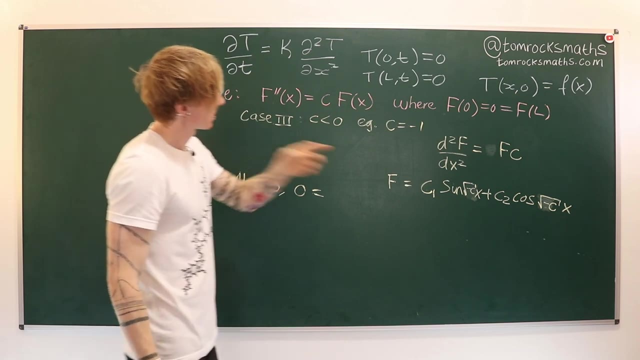 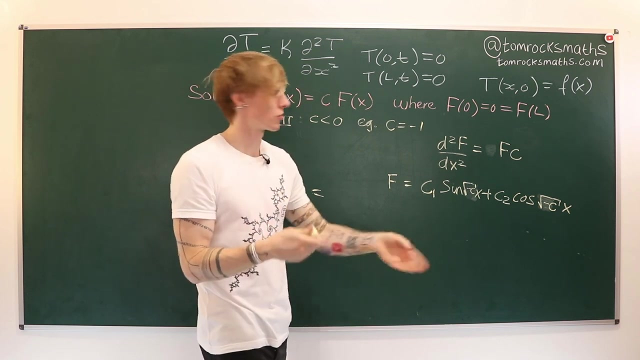 Now we're ready to apply the boundary conditions. So first of all, at x equals 0, we know that 0, our function f has to be equal to C1 times sine of 0. Sine of 0 is 0, so we get no contribution from that. And then cos of 0, well, that's 1, so we 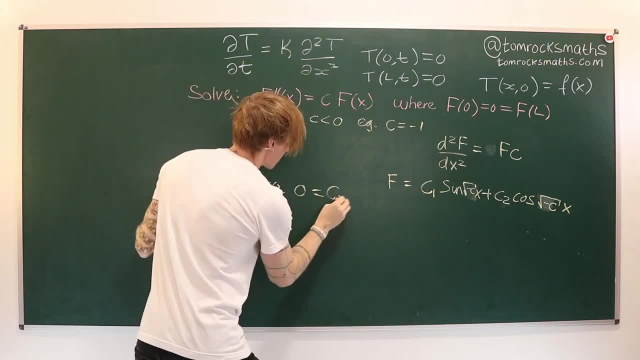 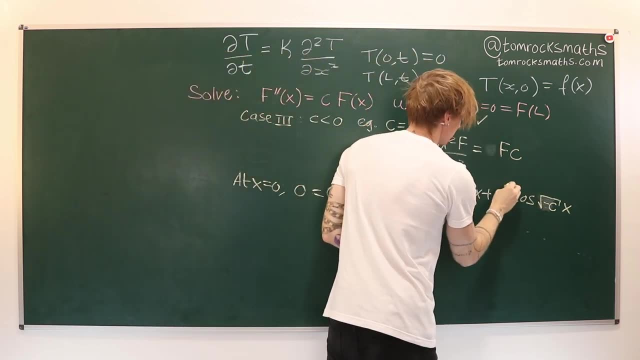 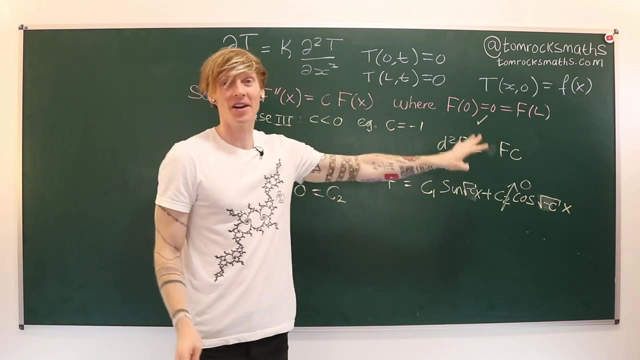 get 1 times C2.. So at x equals 0, we get: C2 must be 0 to satisfy this first boundary condition. So that term there has disappeared. Now hopefully when we apply the second one we don't get that C1 is 0, because then we're back to the 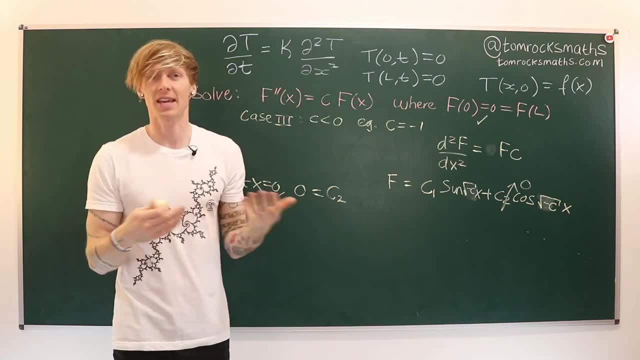 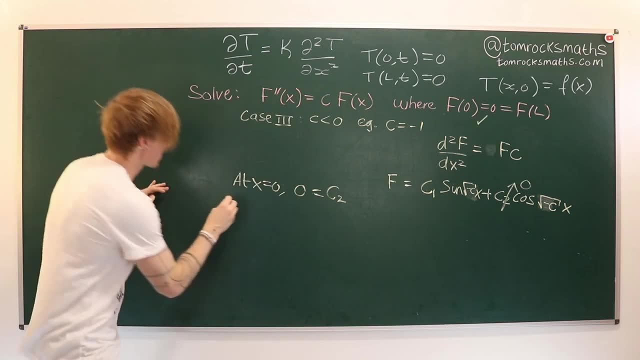 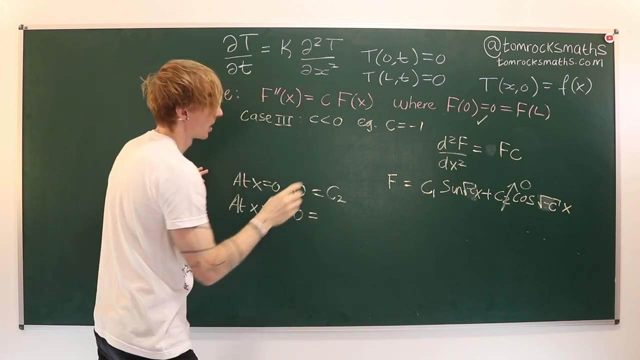 trivial solution, which is the same thing we found in all of the other cases, for positive and 0 C. So let's hope that doesn't happen, But let's apply it anyway. So at x equals L, we need 0, to be equal to c1, so c2 is zero. so the cos terms vanished and what we're left with is c1. 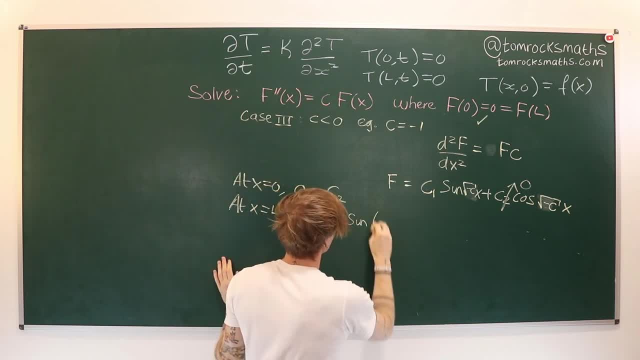 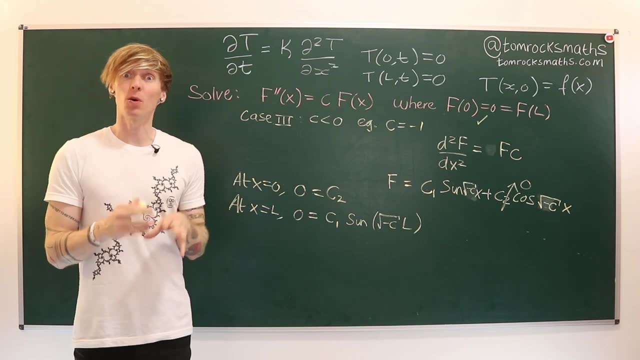 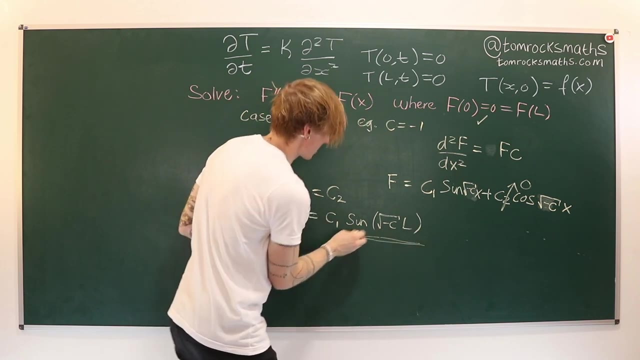 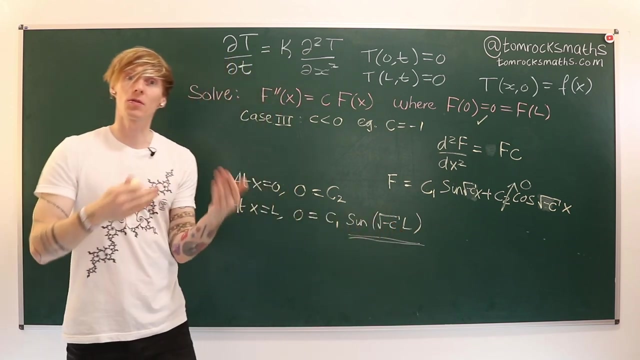 times sine function of the square root of minus c times l. Since we don't want c1 to be zero, then what that leaves us with is trying to make sine of root minus c times l equal to zero. Now l is fixed. it is the length of the rod in the problem. so rather than restricting 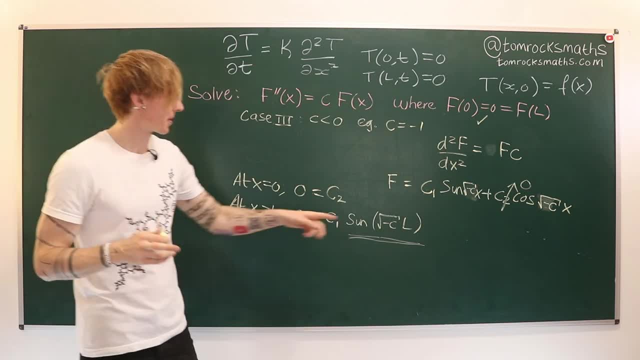 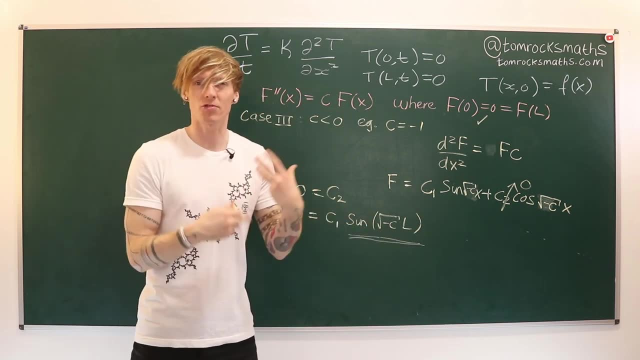 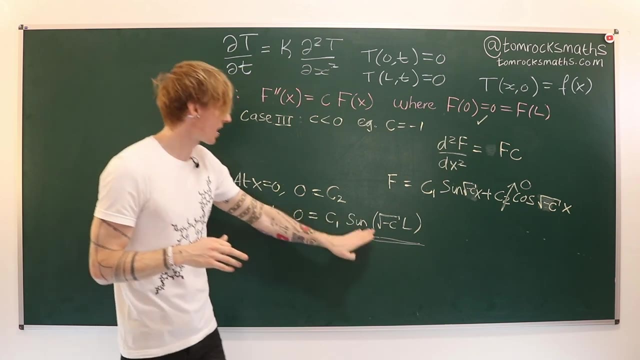 to only certain lengths of rod. what's actually going to happen is we can say this is true for specific values of c, because c was the constant we introduced when looking for separable solution. So what we need to do is look at when the sine function is equal to 0. So if I draw a 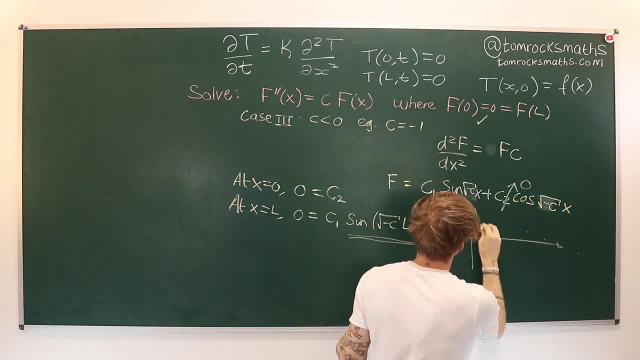 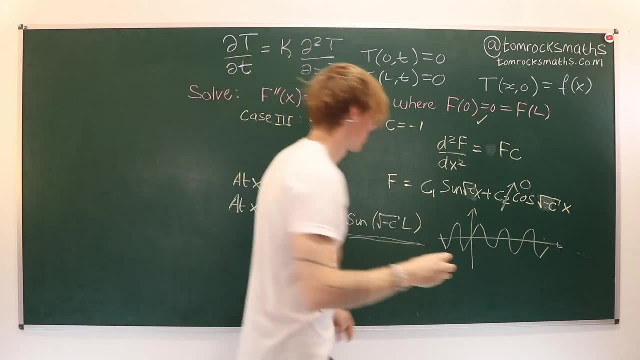 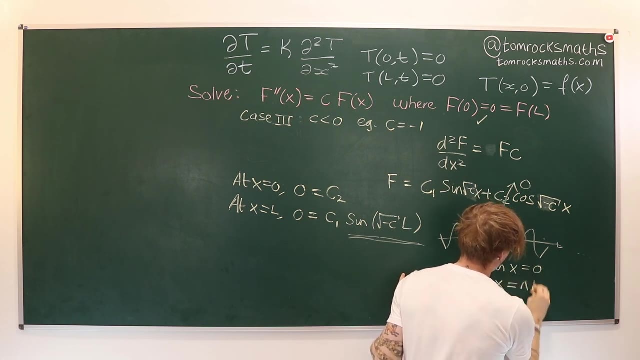 quick graph of sine over here. it's going to go up down, up, down, up down, and it's also going to do the same over here. Then we can see that sine is 0, so sine of x is actually 0 whenever x is an integer multiple of pi. So if n is 0, sine of 0 is 0,. 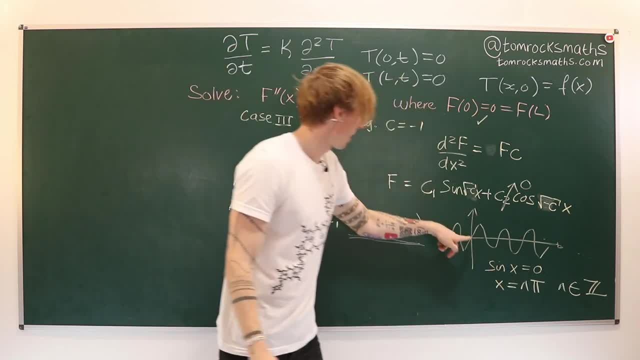 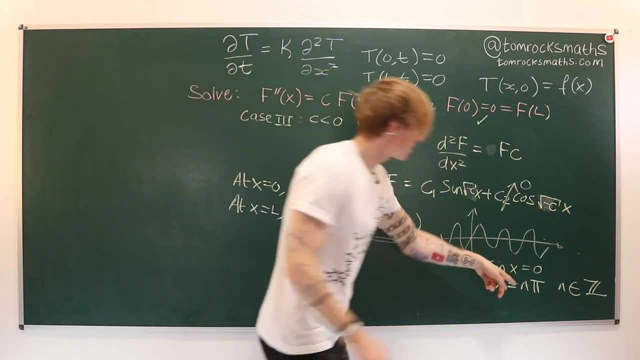 and then it's 0 at pi 2, pi, 3, pi, 4, pi, 5 pi, and also minus pi, minus 2 pi, minus 3 pi, etc. in both directions. So for any integer multiple of pi we can make the sine function 0. 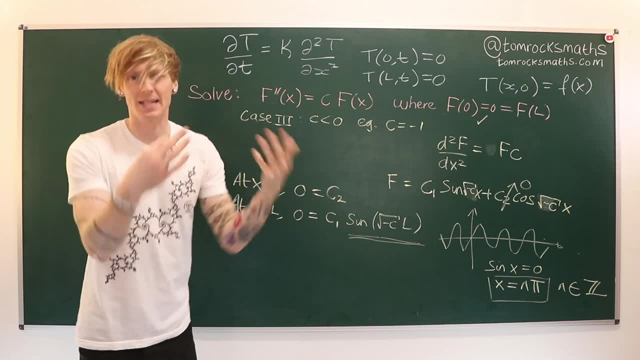 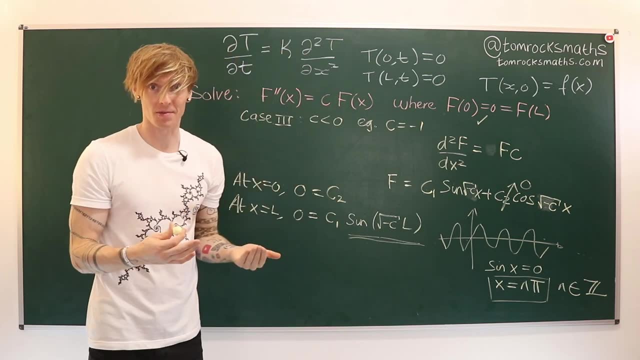 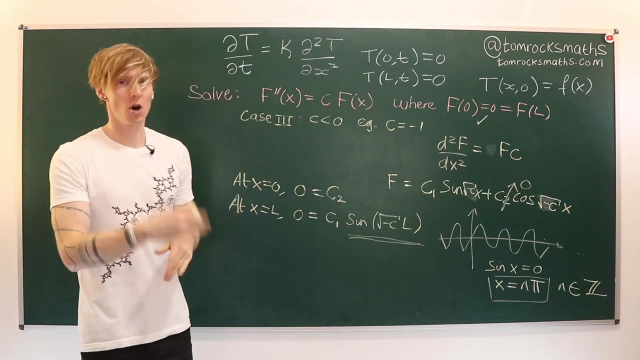 without having to make the constant 0 and therefore getting an identically zero solution. And this is really the key part of this separation of variables type argument for this problem: We restrict the values of c such that we can get a non-trivial solution. 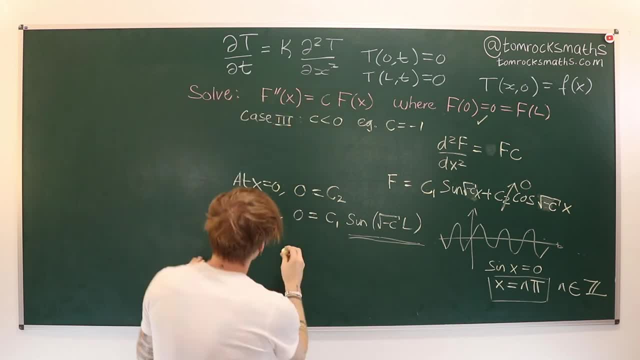 So what that's going to mean here is the square root of minus c times l has to equal n times pi for integer n. Now we can tidy this up a little bit. We can divide by l on both sides and square, and we get that c actually has to be minus n squared, pi squared, divided by l squared. So this: 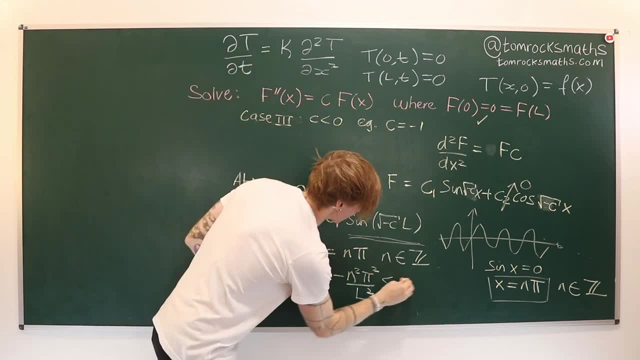 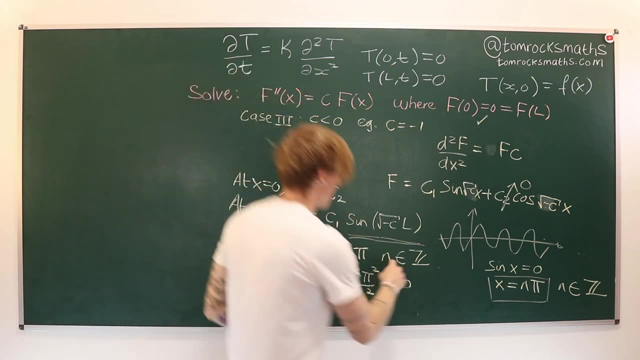 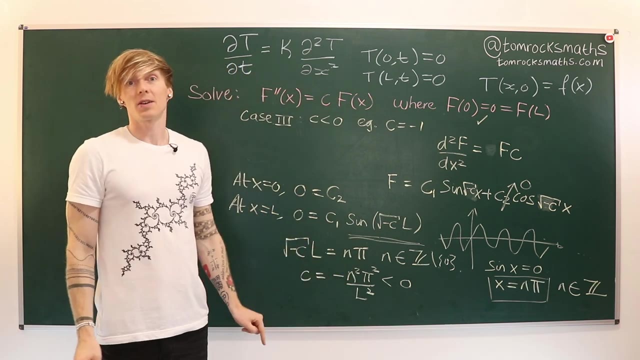 is a clearly negative number. This is definitely less than 0. It actually rules out the case that n is 0. So we need n to belong to z without 0. And in fact, because we are squaring the value of n, it doesn't actually matter whether n is positive or negative. You're going to end up with 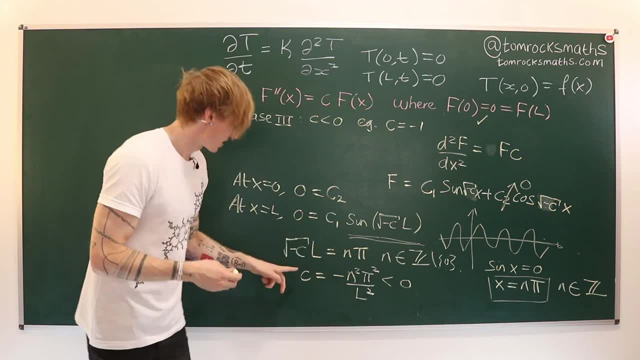 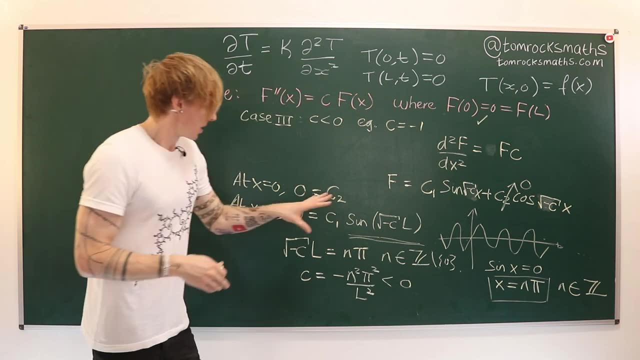 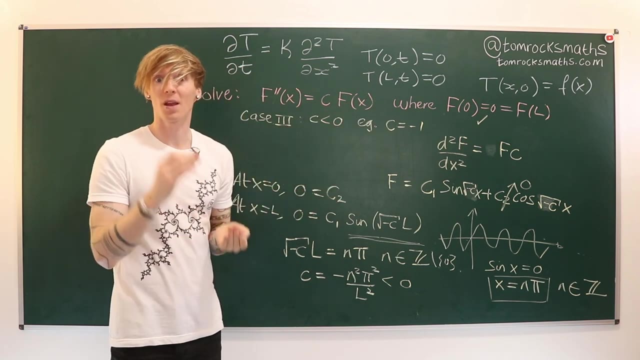 the same solution, Because if n is 2 or minus 2, c being minus n squared, pi squared over l squared, is going to still give you the same value for c. So ultimately, we can say that we have a solution of this form, of this separable form, whenever our constant c is equal to minus n. 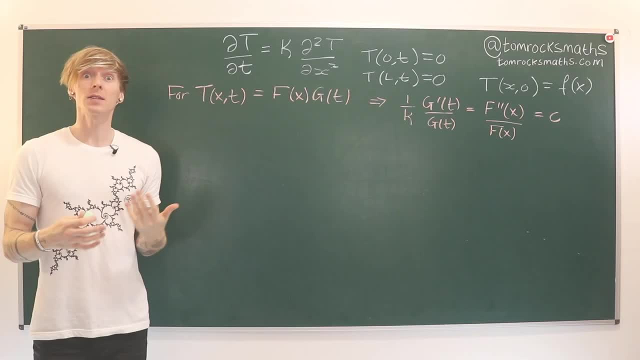 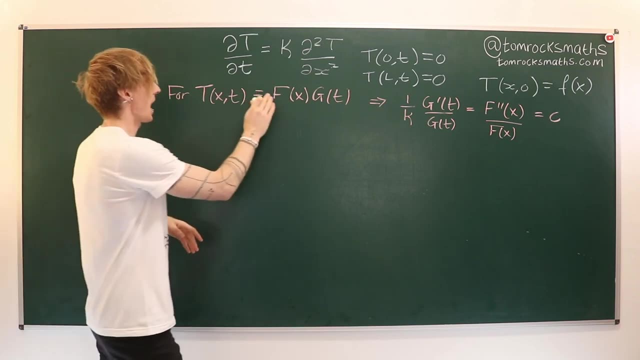 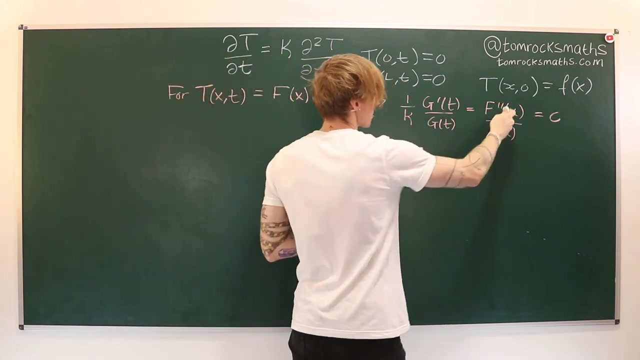 squared, pi squared over l squared. Taking stock of everything we've gone through so far, we started by looking for a separable solution of the form f of x times g of t. We substituted it and said: this is a function of t, this is a function of x. They're equal, They both must. 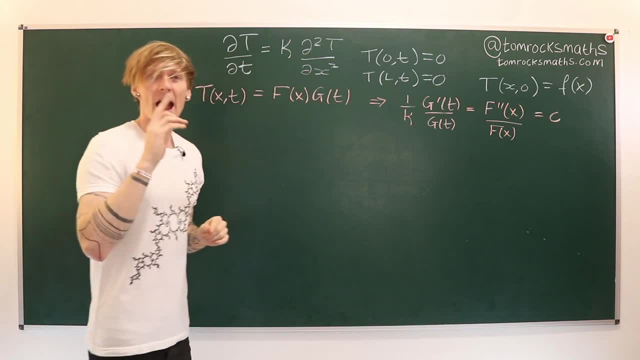 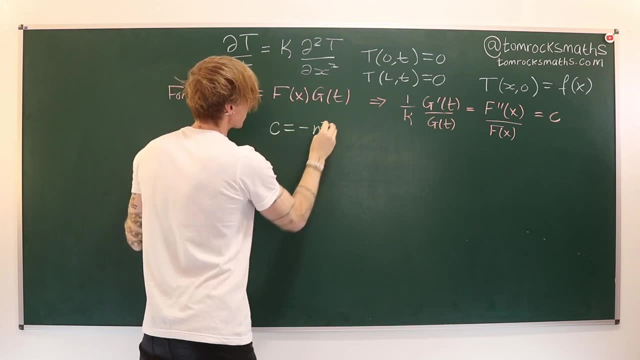 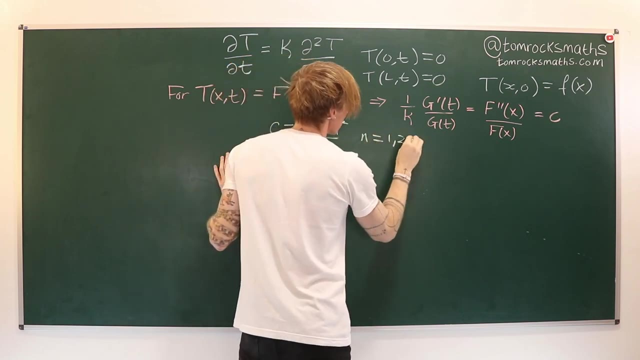 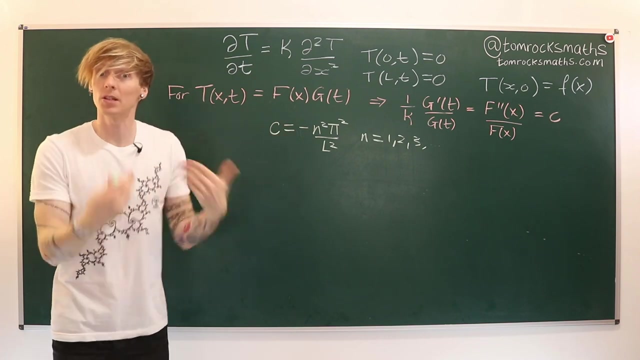 be equal to a constant. Let's call it c, And we just found that the only way this is true is if c is equal to a negative constant, which has to be minus n squared, pi squared divided by l squared, where n can equal 1,, 2,, 3,, all the way up to infinity. Now, in this situation, our solution: 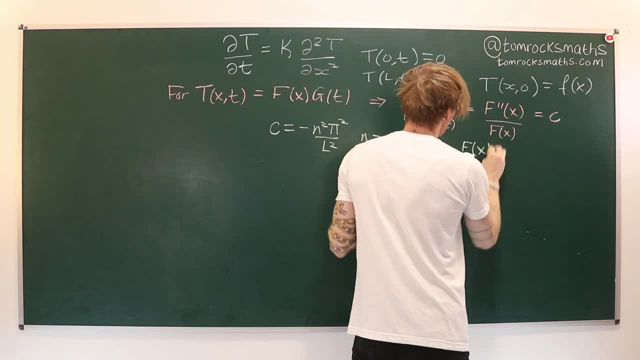 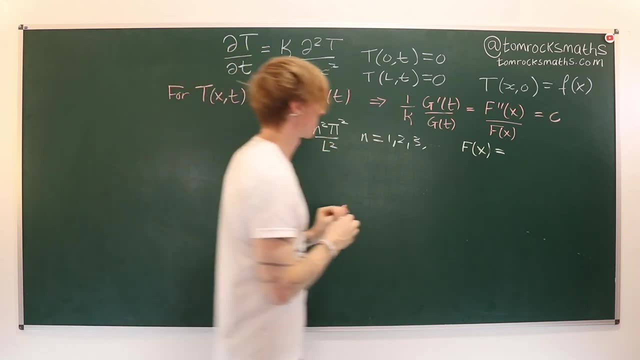 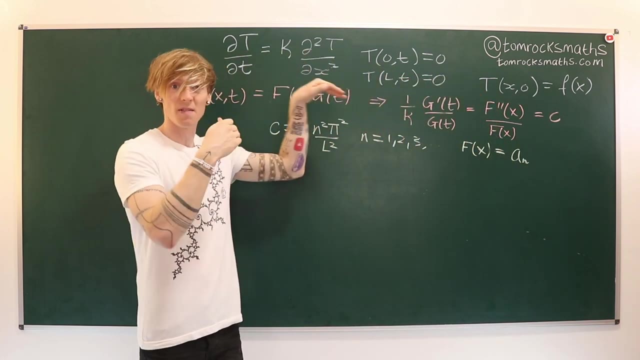 was f of x was equal to a constant which, to help differentiate between the different values of n, I'm going to just put a subscript, So I'm going to call it a subscript n, because it might change depending on the value of n we select. They're all true, of course. a n multiplied by the sine. 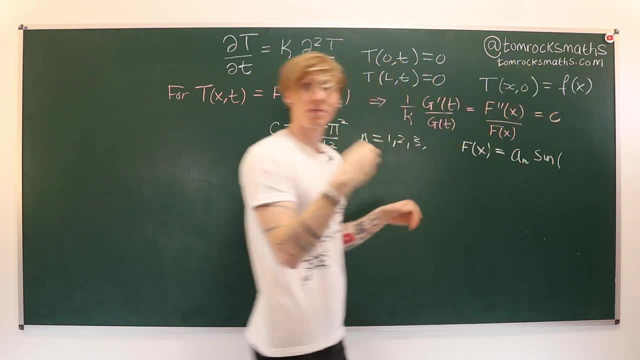 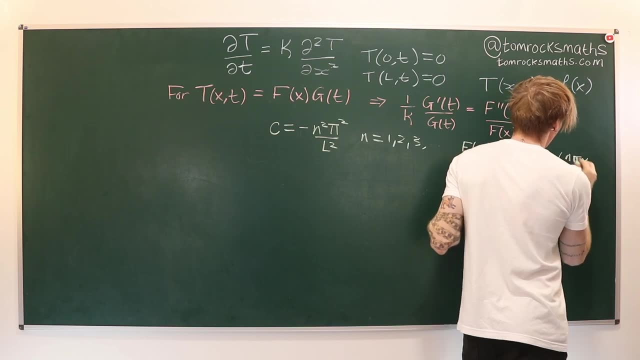 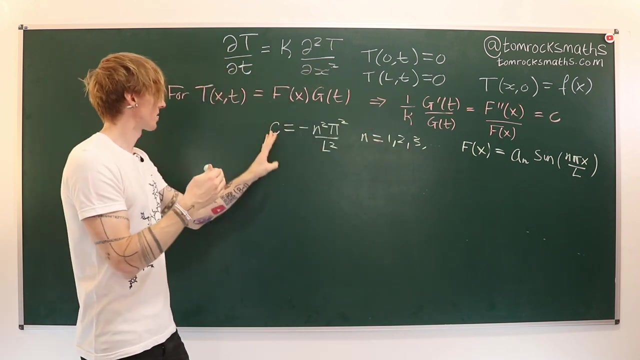 function of the square root of minus c. So that's going to be a square root of minus c. So that's going to be n, pi x over l. So if we fix n, pick a value of n, then this value of c has to be true. 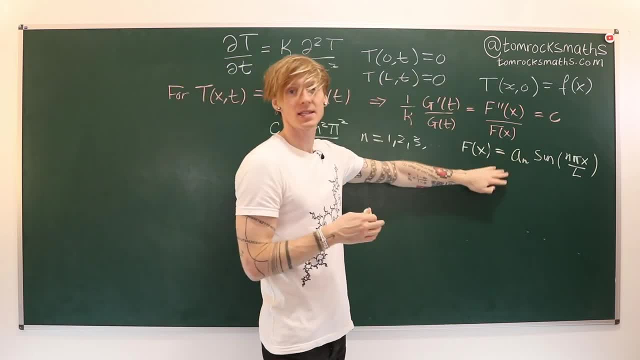 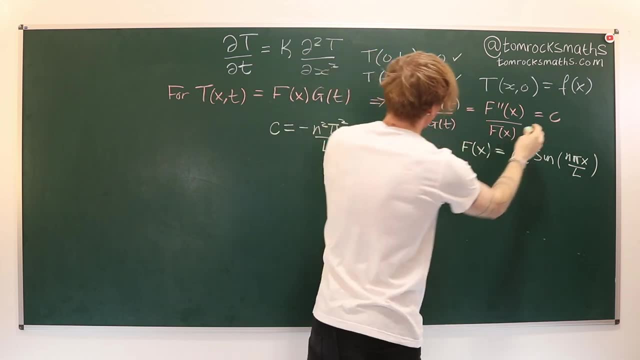 This has to be true to satisfy this equation- and this is our x function that satisfies the two boundary conditions up here and satisfies this equation. So now we can solve the second of our different equations. We're going to solve the second of our different equations. 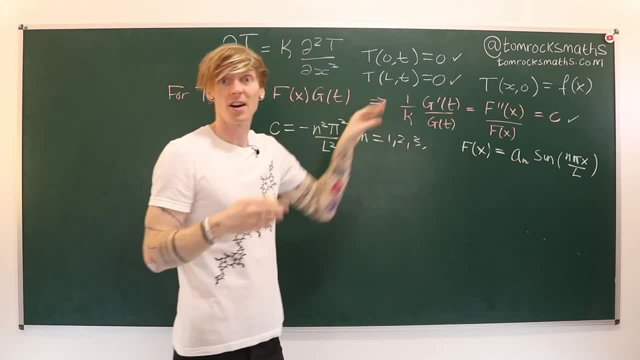 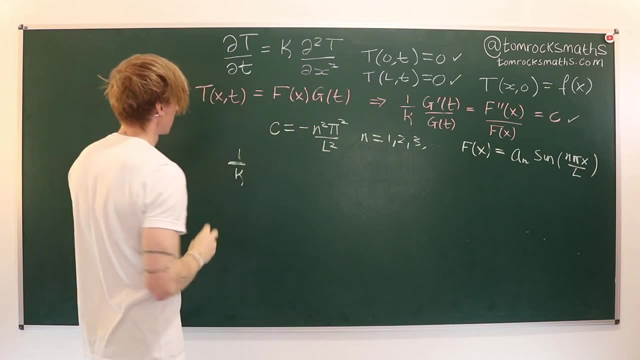 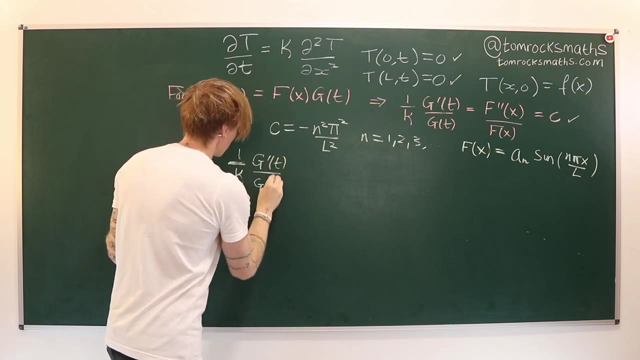 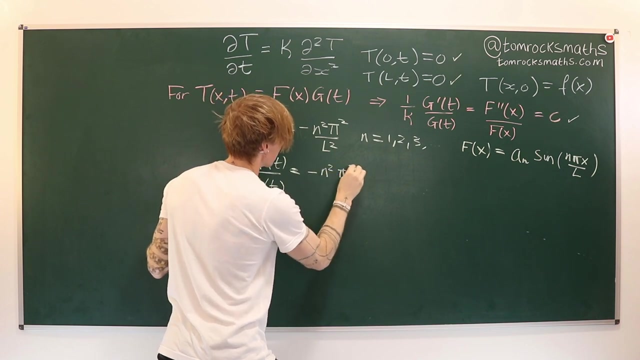 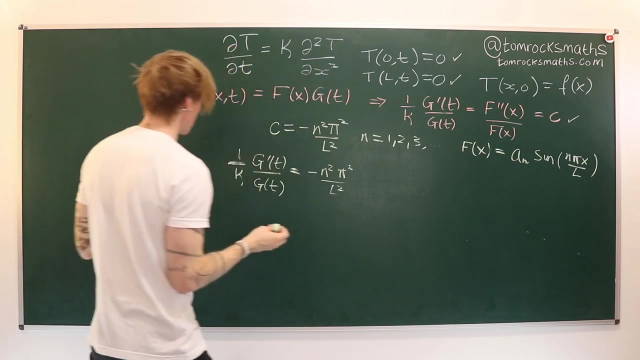 equations, this one for our function of time. So, substituting in, we get 1 over kappa times. the g prime t time derivative divided by g has to equal minus this thing, minus n squared, pi squared over L squared. Now if we multiply through by kappa on both sides, and then what I've got on the left is: 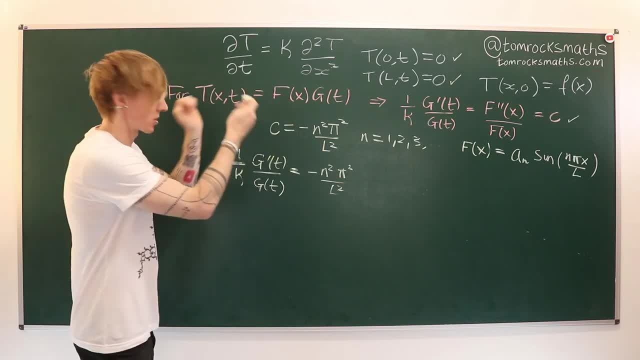 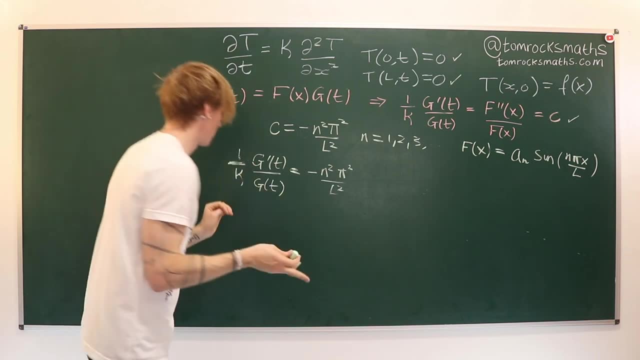 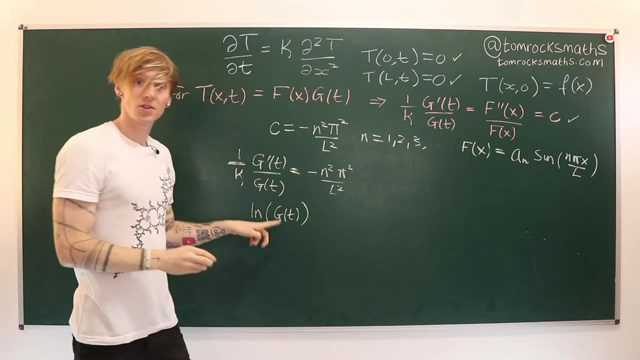 going to actually be a log. So you've got derivative of function divided by function. that is exactly the derivative of log of g of t. So if I just write that out explicitly, we can say the natural log of g of t, just to check differentiate. 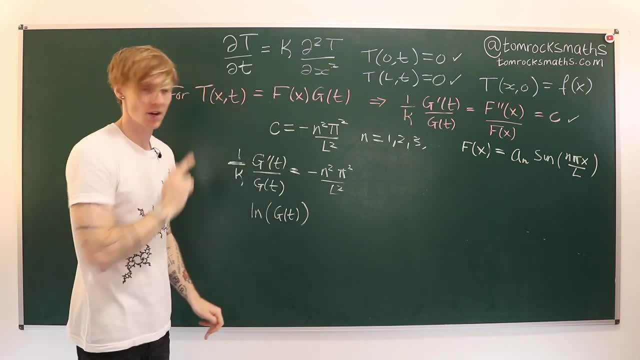 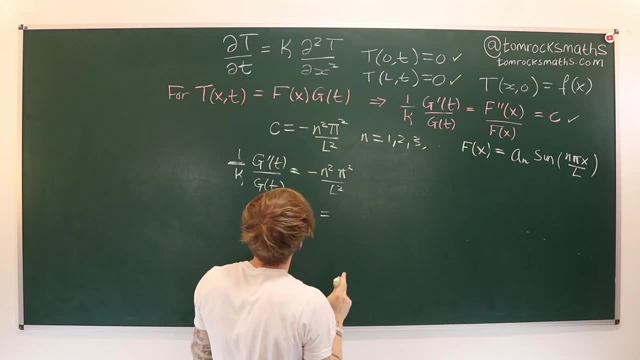 this 1 over g chain rule, so you get a g prime on top. We get that. that has to be equal to this thing integrated with respect to t when we've brought the kappa over. So that's going to be minus n squared pi squared kappa over L squared Integrate. 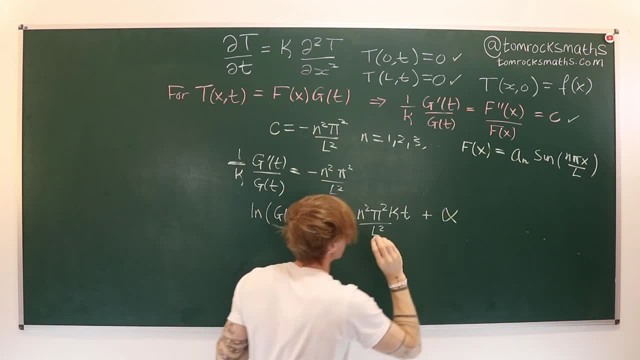 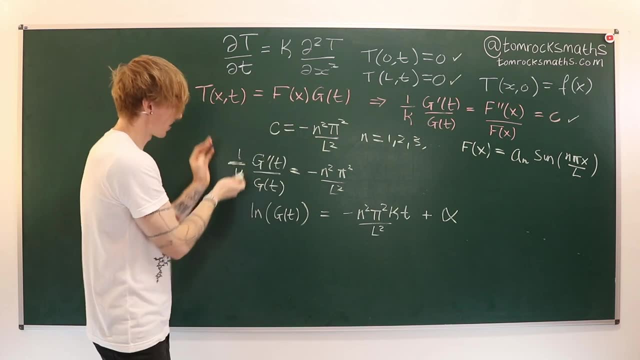 with respect to t and add a constant. I'll call it alpha. So you can either think of this as separation of variables- separating the variables and integrating both sides- or you can spot. this is the log. This differentiates exactly to give you. 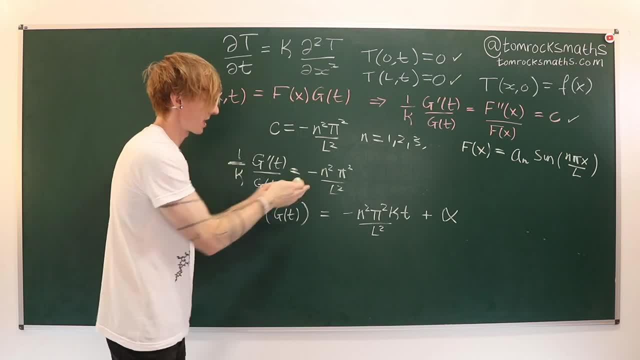 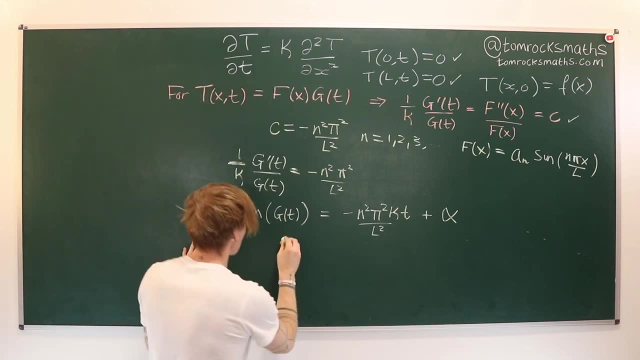 g prime over g. so all I've done, therefore, is integrate both sides with respect to t and just group together those integration constants, Because if I now exponentiate on both sides, I get: g of t is equal to e to the alpha. let's call that b multiplied by. 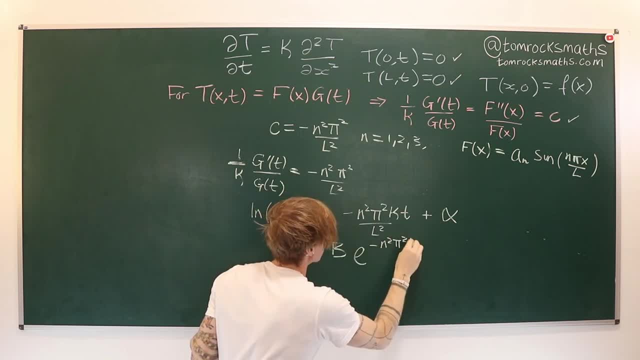 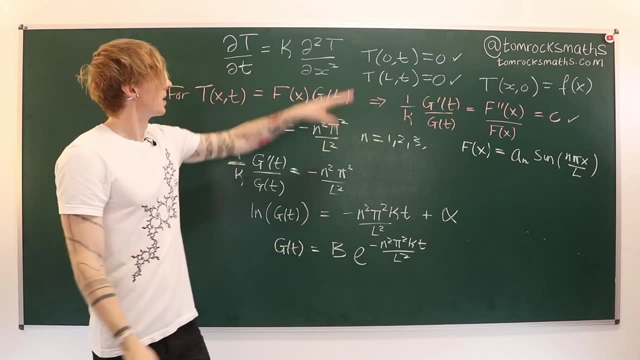 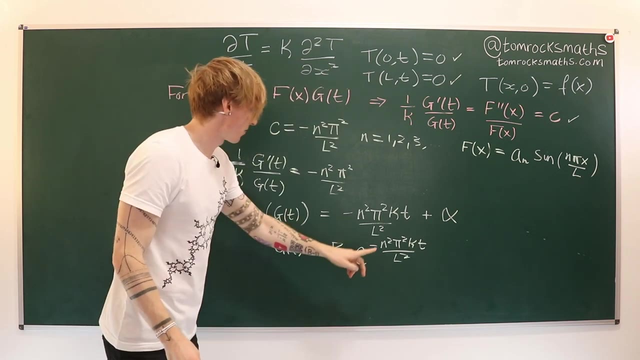 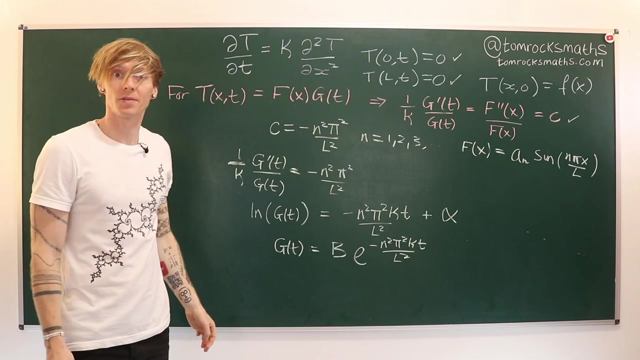 e to the minus n squared, pi squared, kappa t over L squared, And this will satisfy these boundary conditions, because here there's only an x-dependency. so that's completely fine and therefore this also satisfies the equation here when we plugged in our separable solution. So if 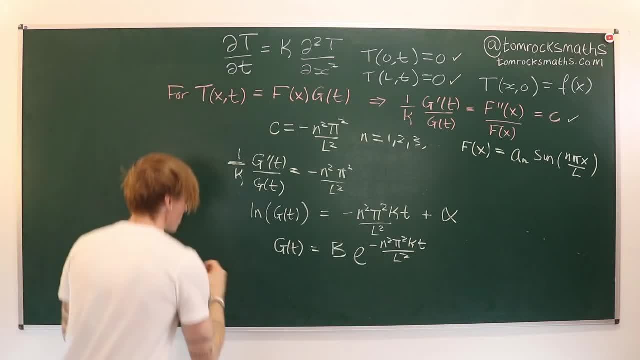 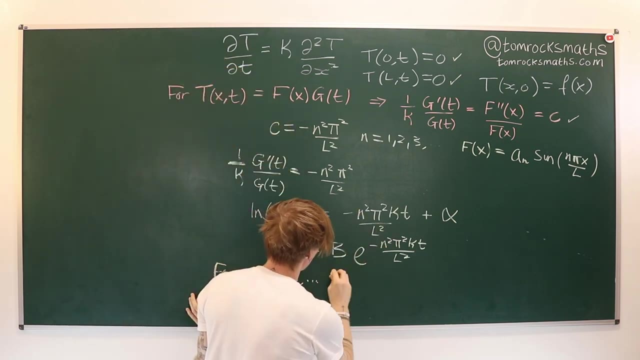 we now put all of this together, we can say our general solution for n equals 1,, 2,, 3, etc. So picking a value of n. we then know our general solution here is f times g. so our solution t of x. t is equal to, if I combine the a, n and the b and call it capital. 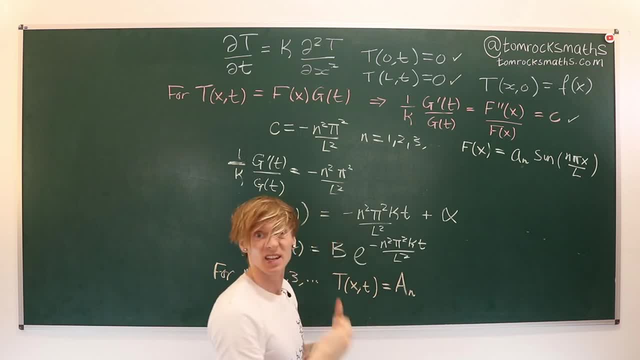 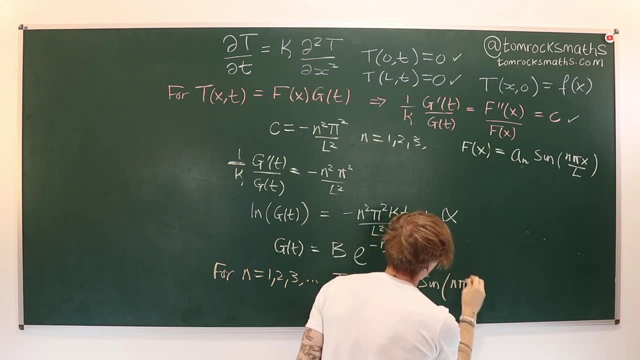 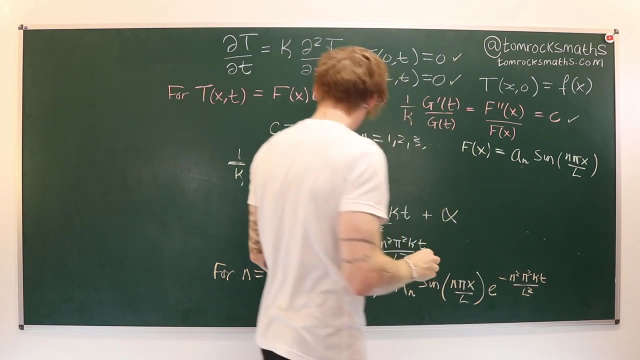 a n, because ultimately it's still an undetermined constant- is equal to a n times sine of n, pi x over L times the exponential e to the minus n squared pi squared kappa t over L divided by L squared. and this function here for any of these values of n, for each value. 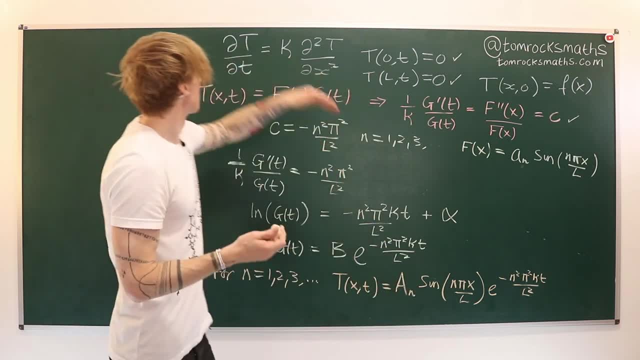 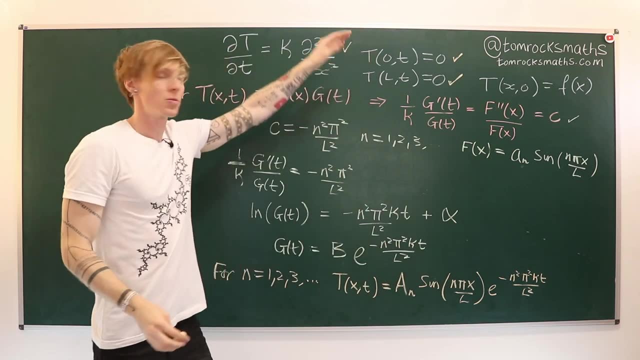 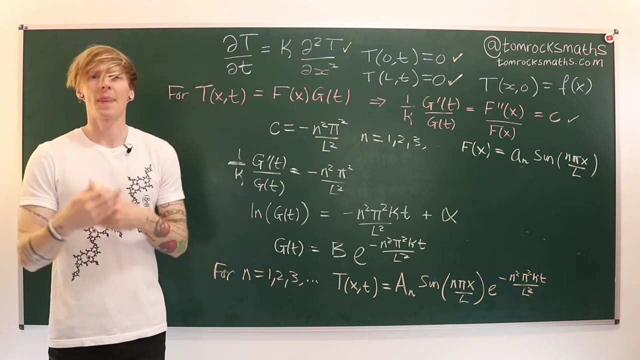 of n individually. this satisfies the original PDE here- and these two boundary conditions for x equals 0, and x equals L. Now there is one final step with our general solution, and that's to do what we call a superposition of each constant. 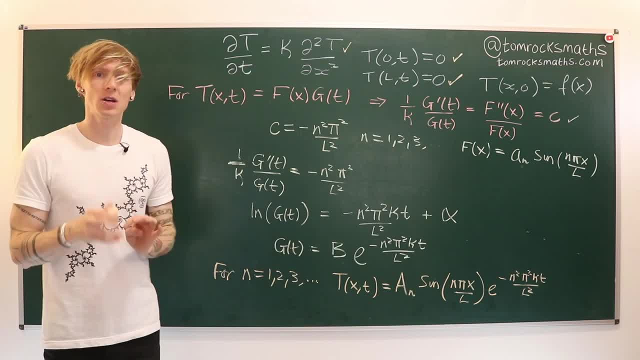 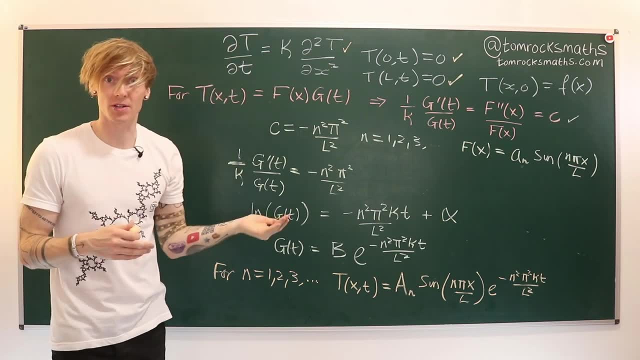 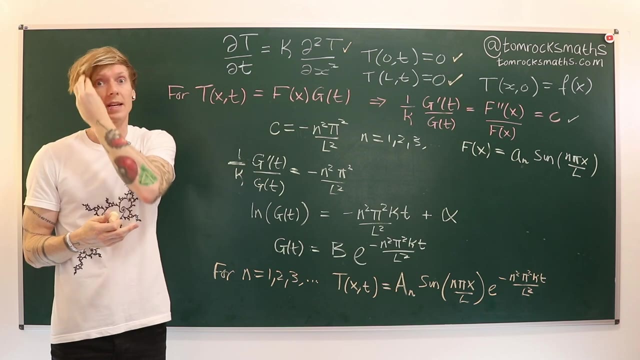 these individual solutions Now, because the heat equation is linear. what this means is, if you have one solution to the heat equation, let's call it solution A, and then you have a second, different solution, let's call it solution B, also satisfying the same problem. then, if you take 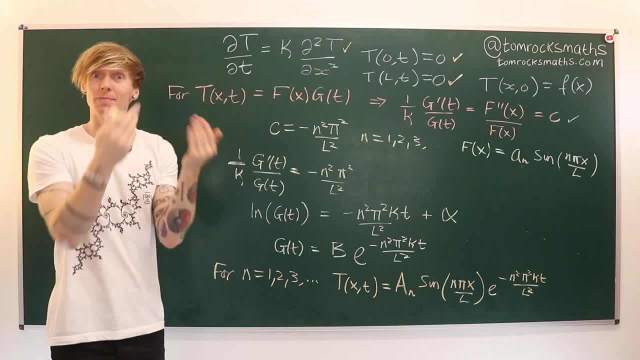 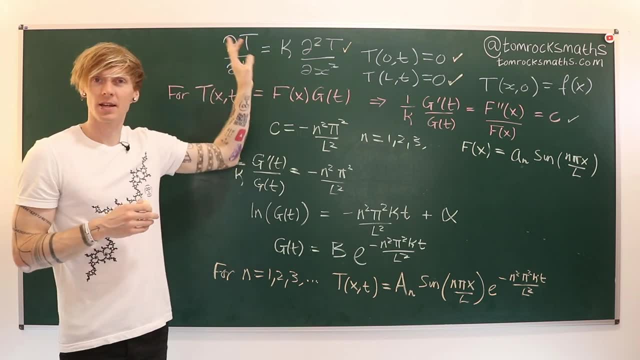 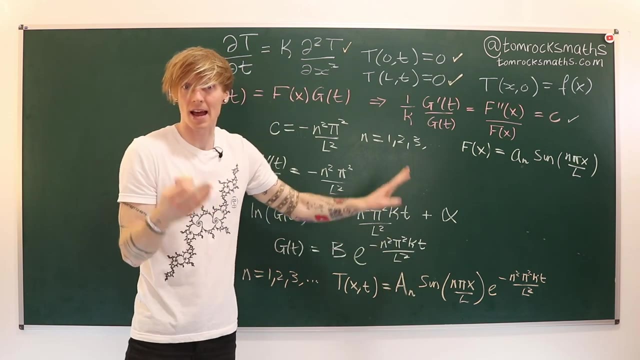 A and B and add them together, so your solution is now A plus B. then that summation of your two valid solutions is also a valid solution. And if you don't believe me, you can check this. take one value of n in here. fix n at any value you want from our allowed list, sub it in. see that. 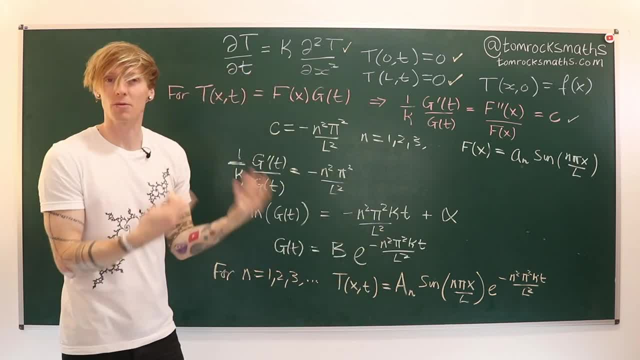 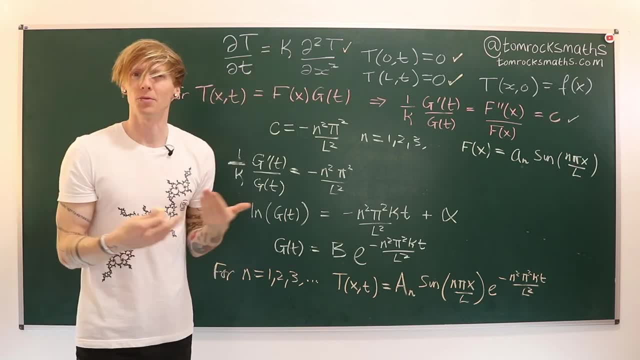 it works. take another different value, sub it in, see that it works, add the two together, substitute in that sum and then you have a solution. So if you take the sum into here and you'll see that everything still works Now, just because it's linear for those two solutions. 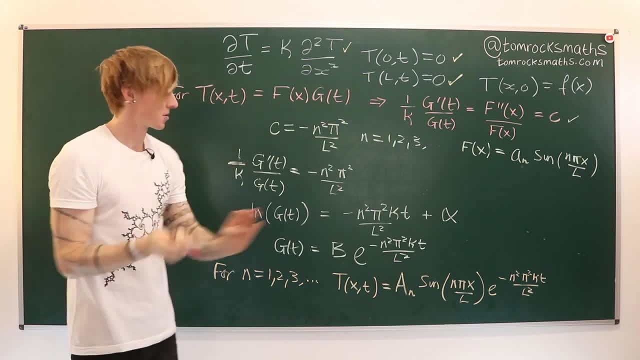 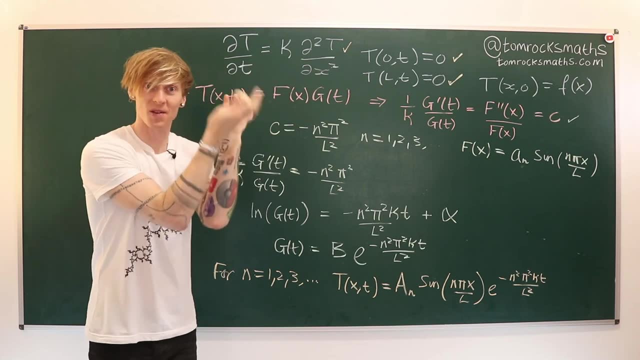 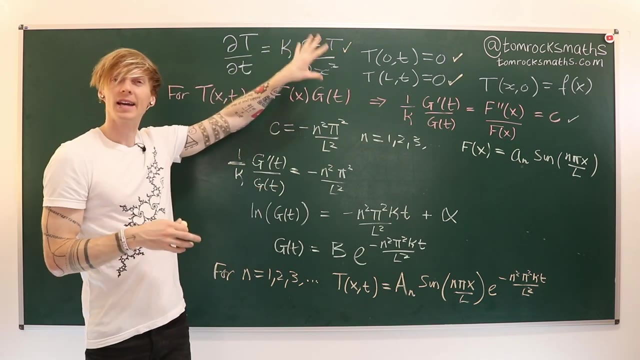 we then get a new solution which has two pieces, so then we can say, okay, that's now a valid solution. let's take another third solution and add together the first two that are now a valid solution, plus the third one, and suddenly we've got the sum of three solutions also satisfying the same problem. 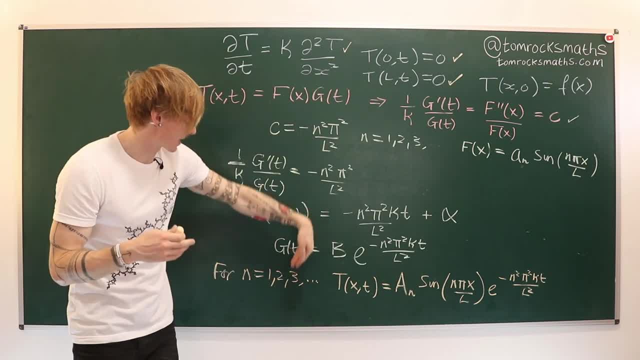 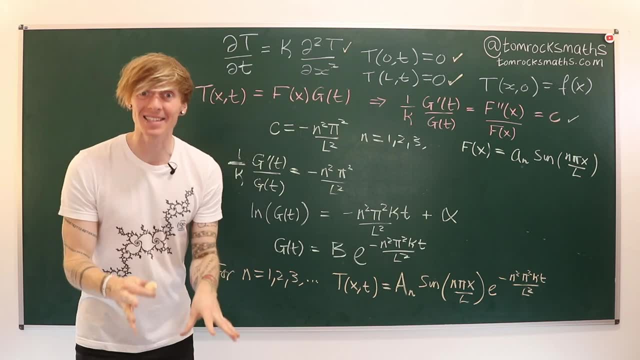 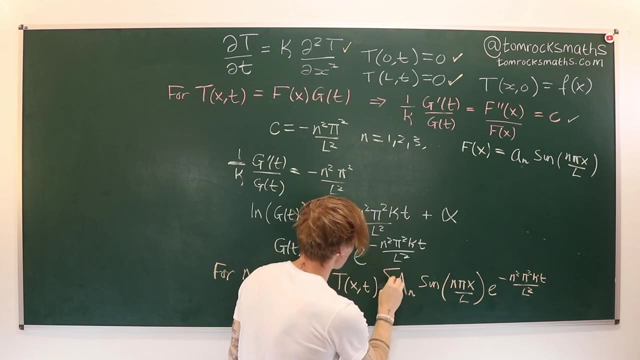 And we can continue like this. We can just keep adding each one of these solutions for each individual value of n. So doing exactly this, we can say that our true general solution is in fact going to be equal to the sum from n- equals 1 to infinity- of each of these valid solutions which we've written down. 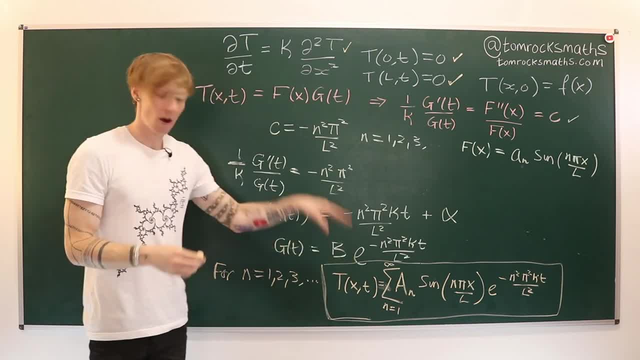 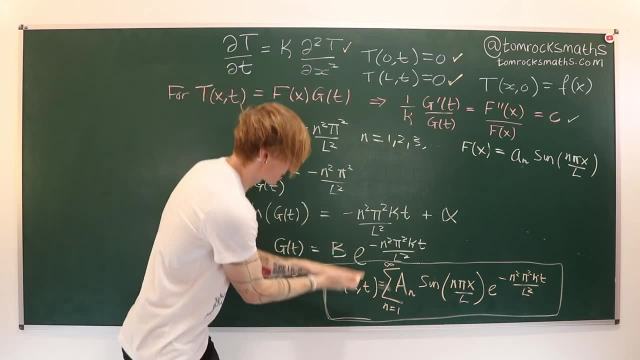 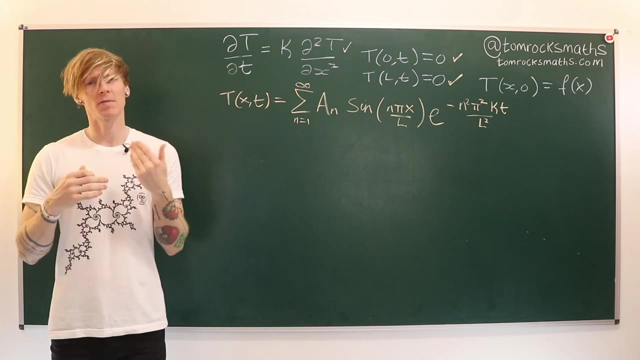 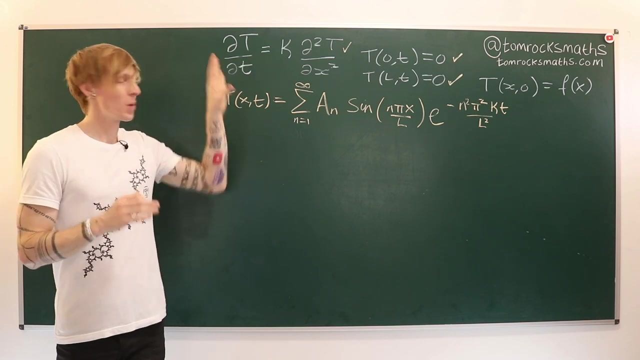 here. So this is our superposition of all of these individual solutions. We can add them all together and create this infinite sum, and this satisfies our original heat equation. Now, the eagle-eyed amongst you may have noticed that we haven't actually yet completely solved the problem. We looked for a separable solution. 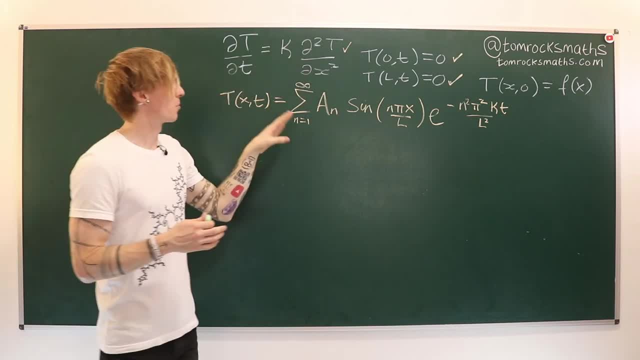 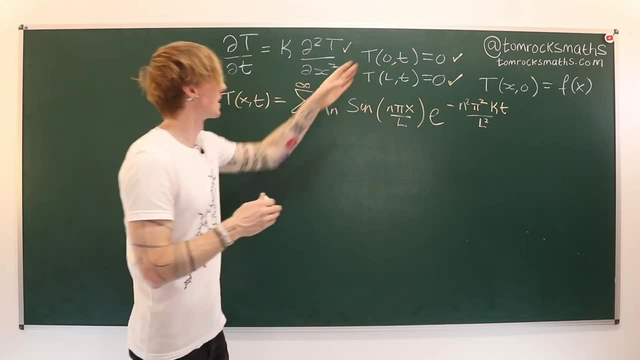 to our original PDE and we found this And we know that this satisfies both of our boundary conditions up here, and if you don't believe me, you can sub them in and check. You will indeed get 0 when x is 0 and x is out. Now the condition we haven't yet satisfied. 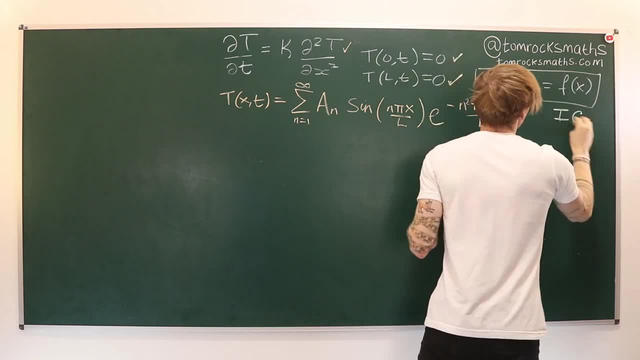 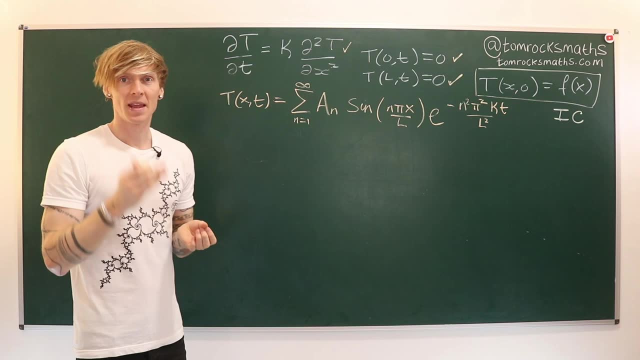 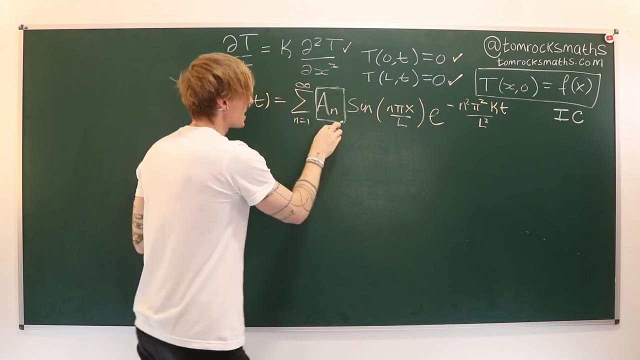 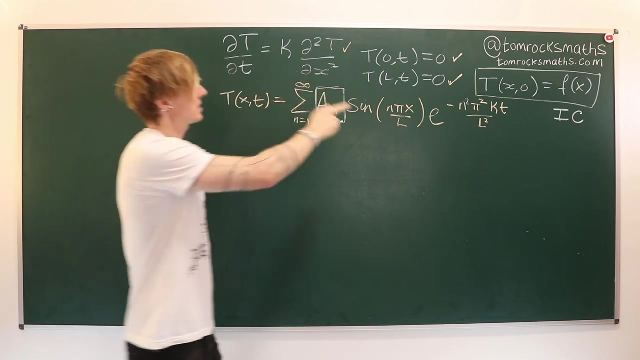 is the initial condition over here, the IC, the initial part of the IBVP, initial boundary value problem, And it's this that's actually going to help us determine what these coefficients a, n, have, in order to complete the full solution to the problem. Now this tells us at: t equals 0. 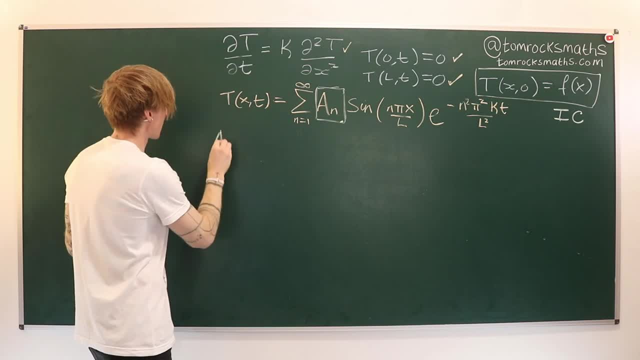 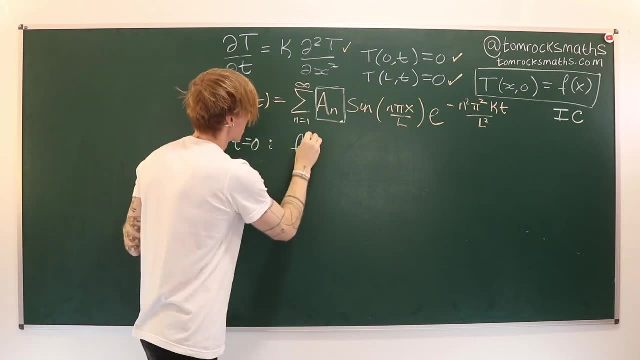 this must be equal to f of x. So if we sub in, so if I say at t equals 0, we need to satisfy This becomes f of x. so we need f of x to be equal to the sum from: n equals 1 to infinity. 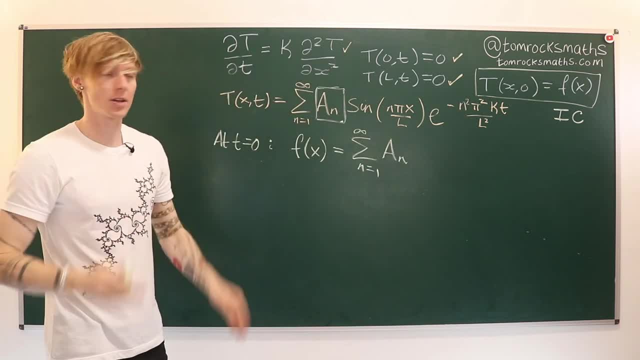 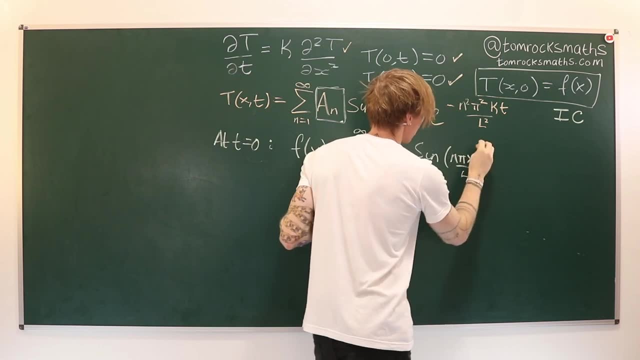 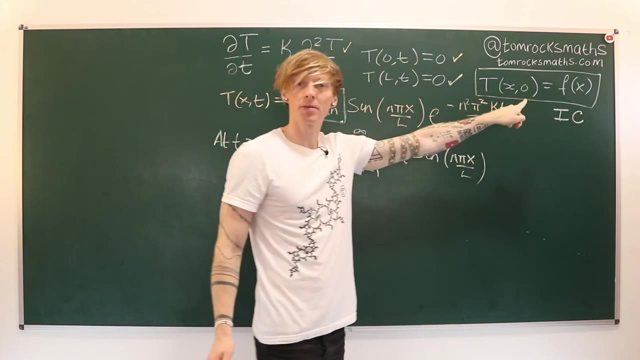 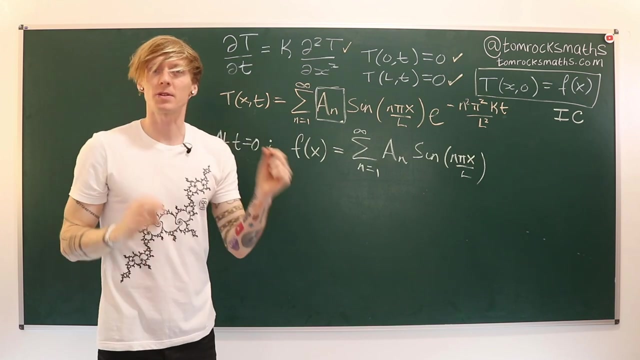 of these constants, a, n, as yet undetermined times, sine of n, pi, x, over l, And now we've got this exponential term, but t is equal to 0. So if I substitute in t equals 0, here I get e to the 0, and e to the power of 0 is 1.. So there's nothing else here. So what we? 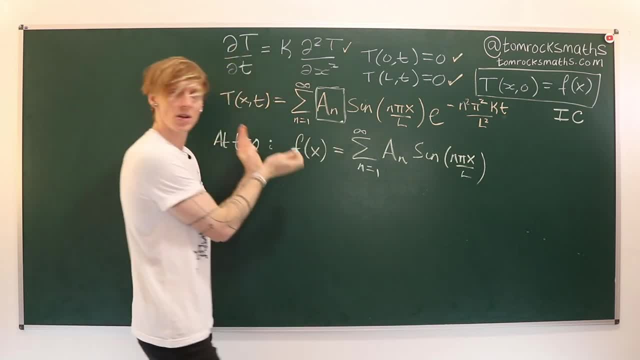 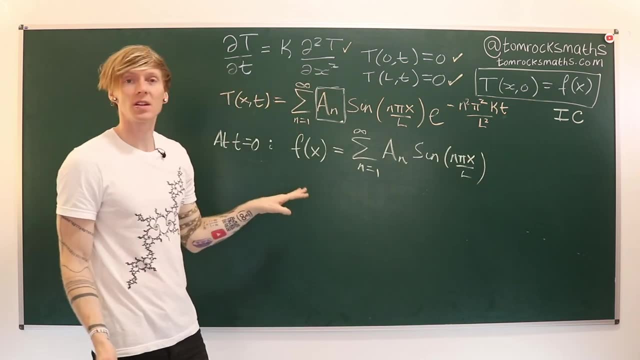 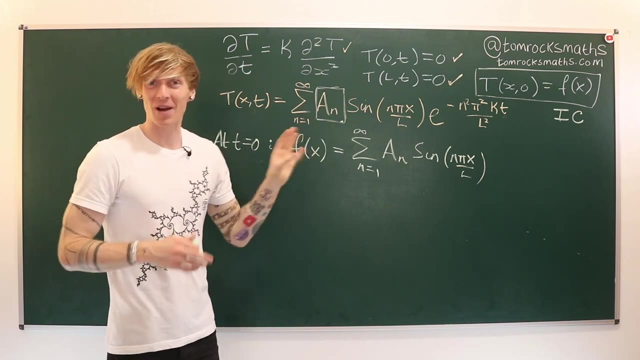 actually have to solve is that we need to solve the problem. So what we actually have to solve is our given initial temperature distribution. f of x has to be expressed as this infinite sine series. Now some of you watching may have realized where this is going. We need to take a. 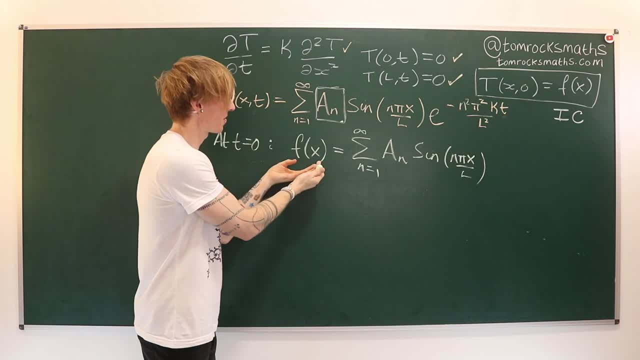 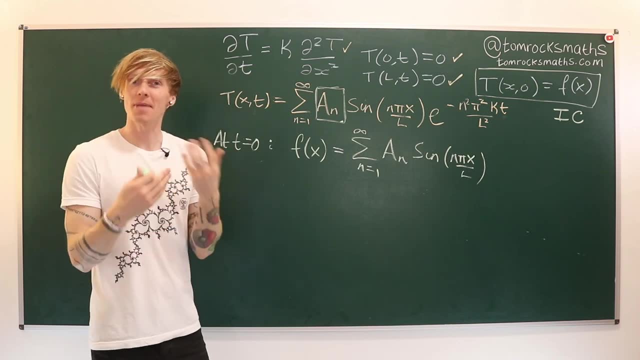 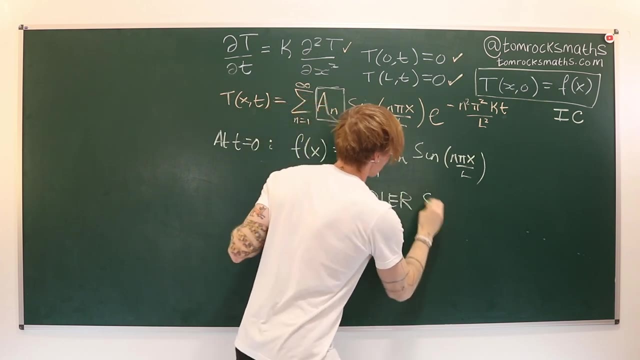 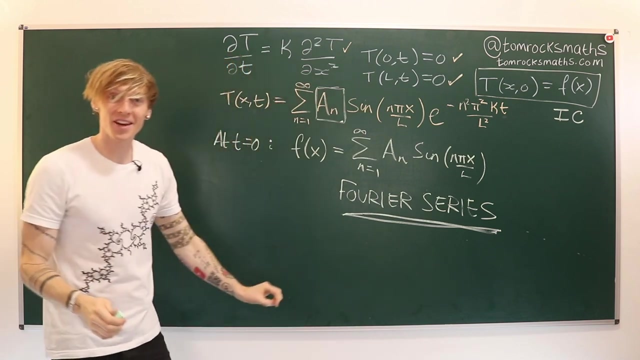 hopefully well-behaved- continuous function f and express it as an infinite series of sine functions, And this is exactly the method of Fourier series. So this, as you may have guessed, is going to be the topic of the next video in the Oxford Calculus series. We've reached a nice point where 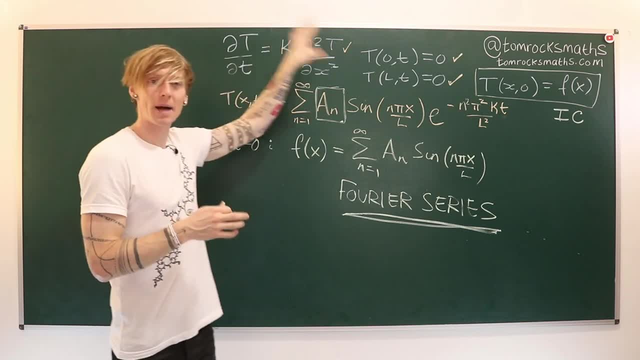 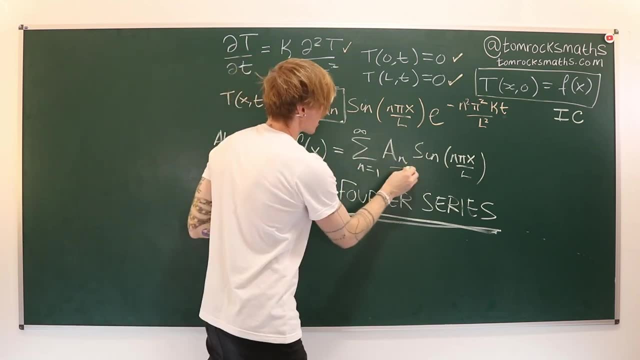 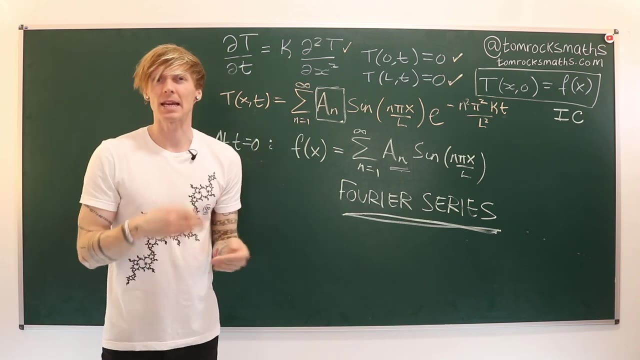 we have a general solution to the initial boundary value problem of the one-dimensional heat equation. All that's left is to determine the coefficients a- n. but in order to do that, we need the technique of Fourier series, which I will be explaining in the next video in this series. As a final note, and this will be: 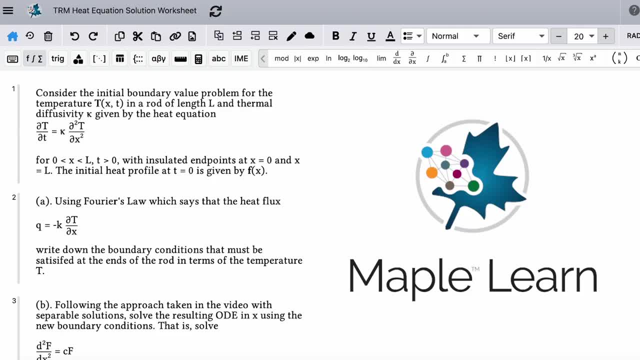 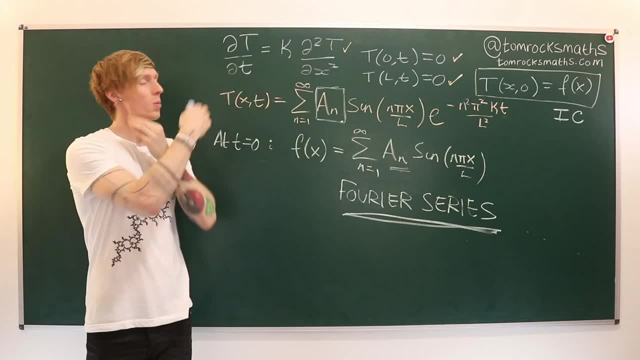 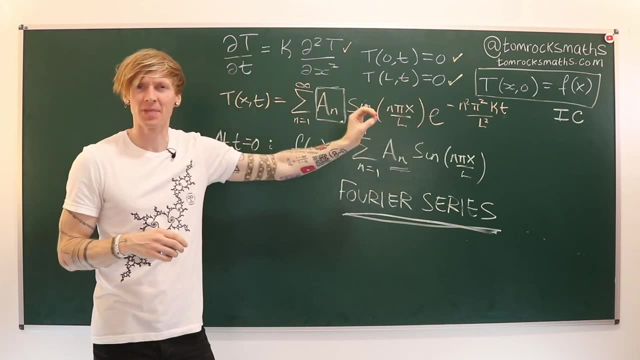 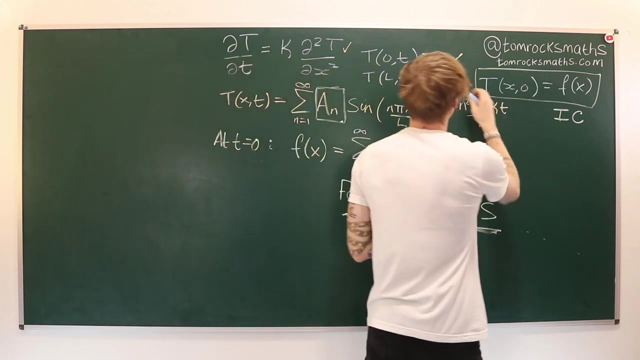 very helpful for the accompanying MapleLearn worksheet which goes along with this video and is linked in the video description. what we've solved here was for a rod with zero temperature at the end points. However, a slightly more realistic example perhaps would be to say that what we 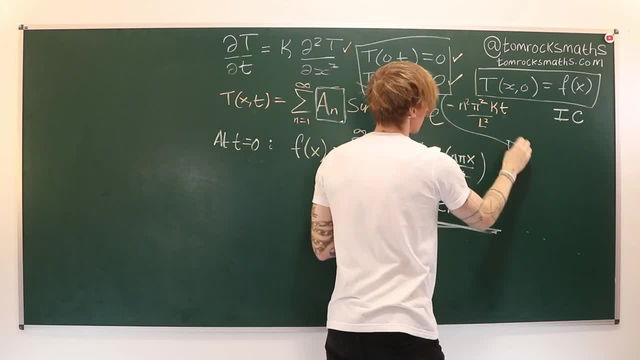 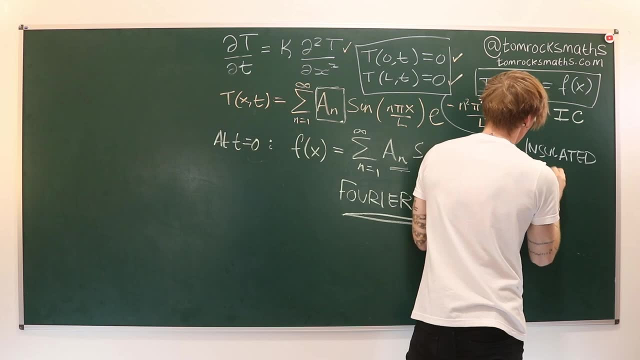 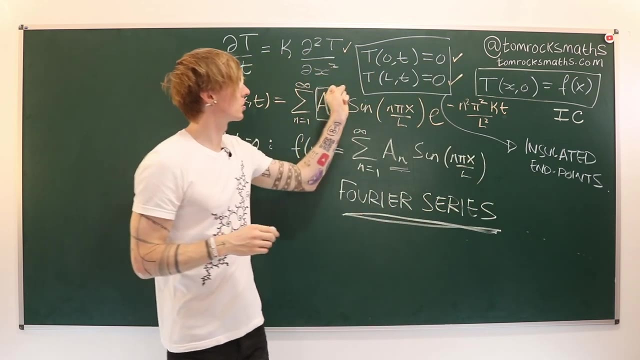 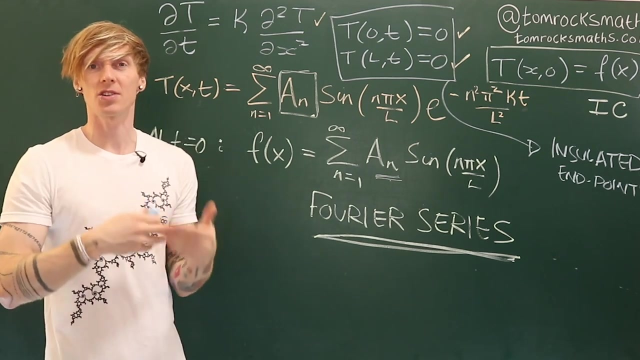 want instead placing these is to have insulated end points. So that's going to mean that there is no heat flux at x equals naught and x equals L. Using Fourier's law, this tells us that the boundary conditions we need to satisfy for an insulated rod are, in fact, that: 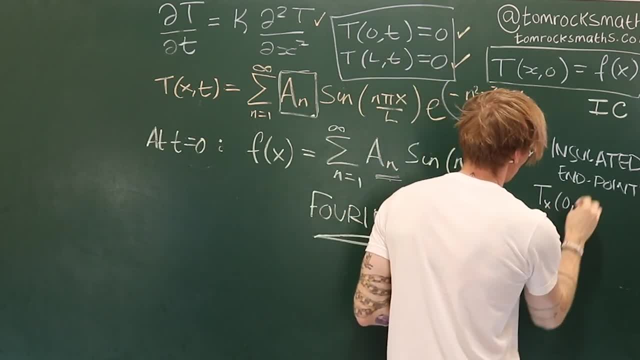 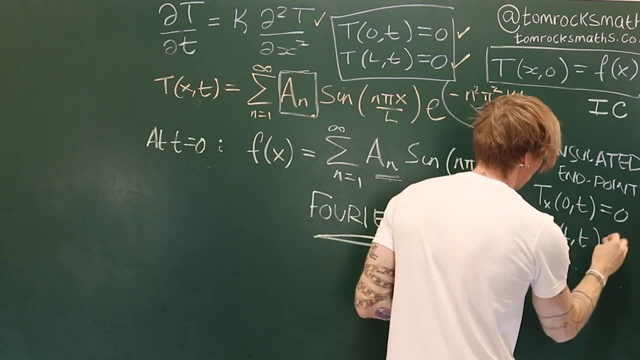 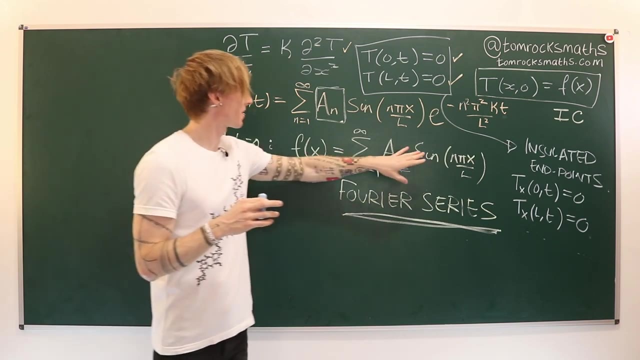 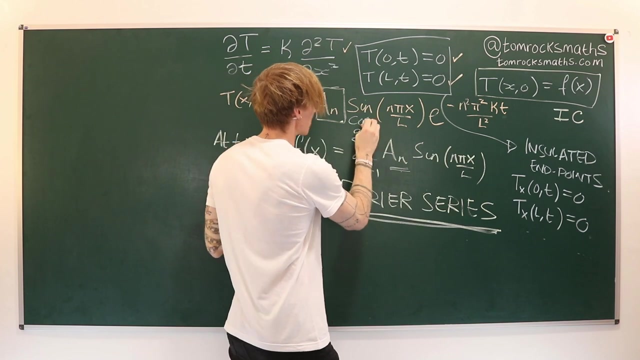 the x derivative at x equals naught must be 0, and the x derivative at x equals L must also be 0. Now what this means for our general solution is, in fact, that instead of having sine functions inside our infinite series, we actually end up with cos in both of these situations. Now the steps of this. 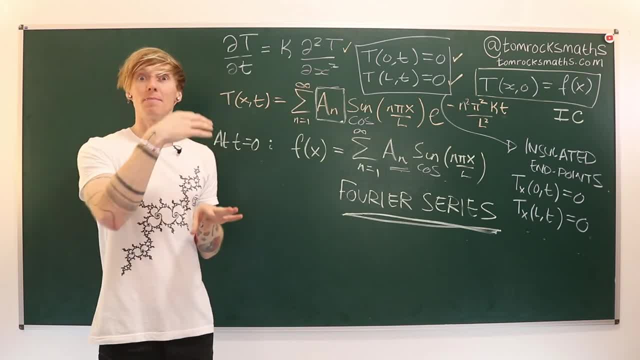 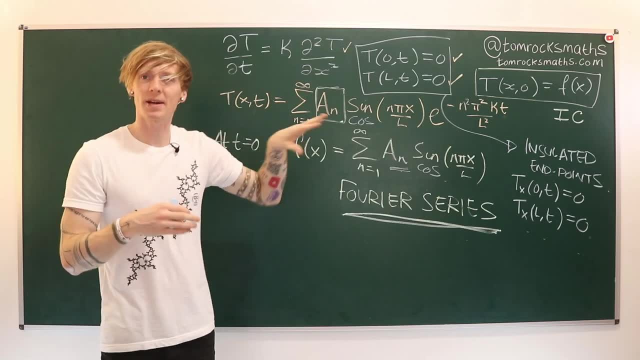 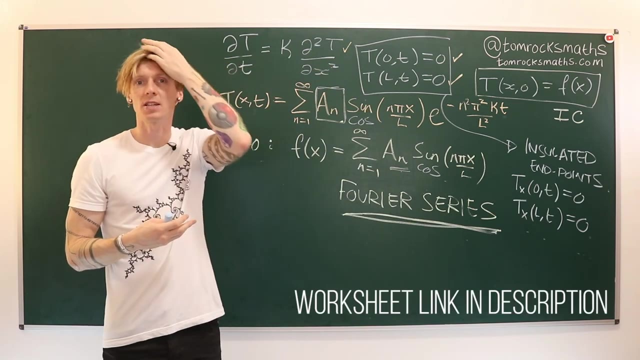 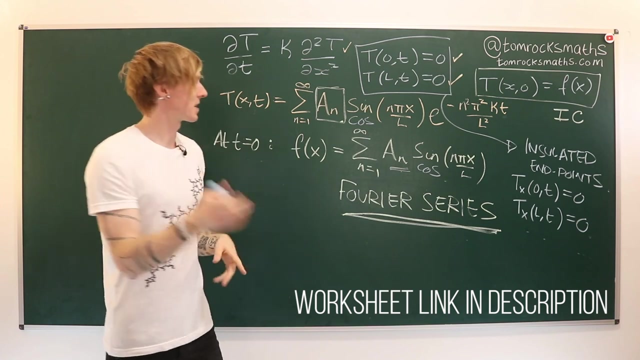 are actually outlined in detail in the MapleLearn worksheet which, as I said, accompanies this video. We will go through step by step how to derive these boundary conditions from the information of an insulated rod, and then how that affects the solution. following the solution, The same steps we've done here, but instead ending up with the cos series. 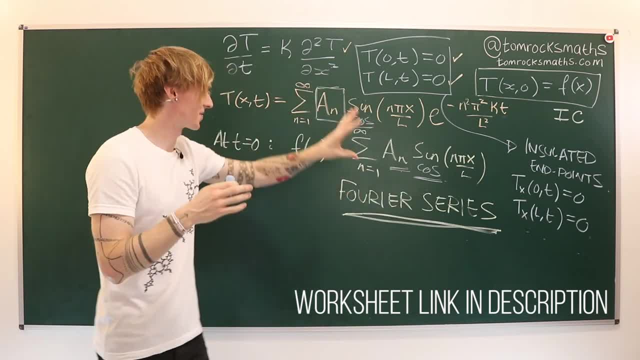 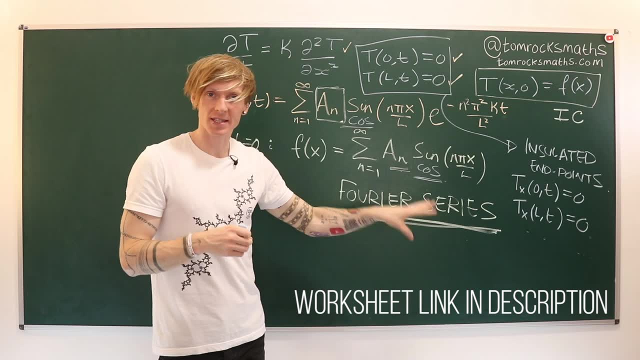 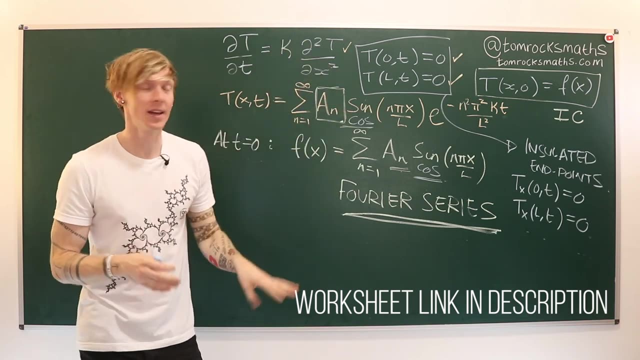 Fourier series will still apply, because Fourier series allow us to rewrite a function f as either an infinite sine series, an infinite cos series or, in some cases, a sum of both. So the same technique will still work, but in order to see all of the details, I do recommend checking out the MapleLearn worksheet. 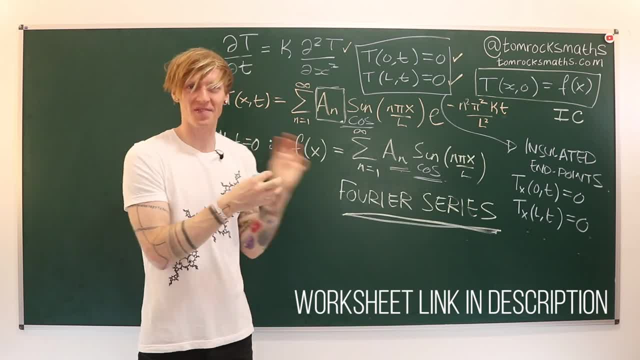 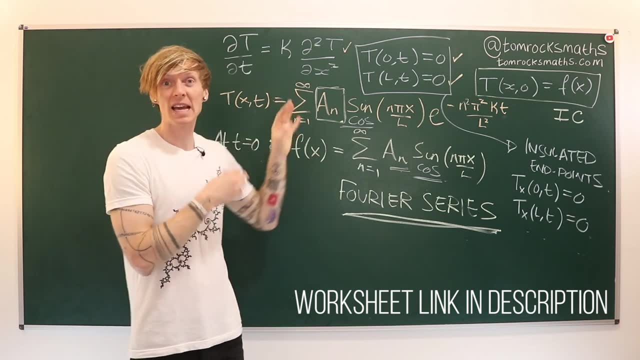 It's, I think, a very useful tool. I think very interesting to see how this affects the problem, but it's also a great way to practice and to check that you really do understand what we've covered in the video. Thank you everyone for watching. Please do remember to. 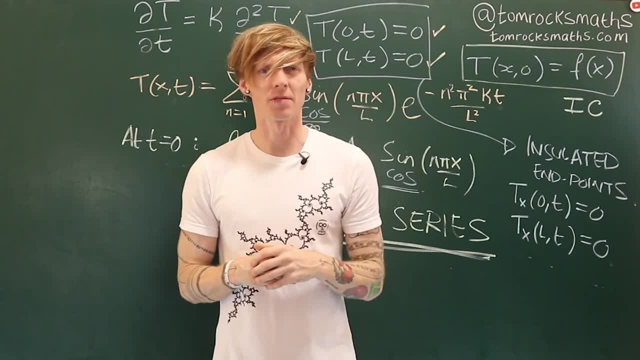 subscribe if you've enjoyed the video and I'll see you all soon. Take care.